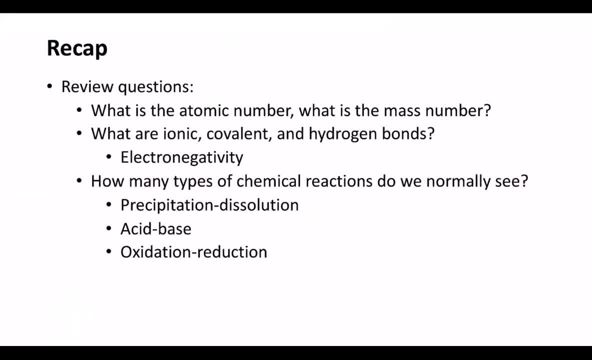 We mainly reviewed some basic properties of the elements or of molecules. So, for example, we talked about what is the atomic number, what is the mass number or what is the atomic weight, right? So we mentioned the atomic weight. is the situation. 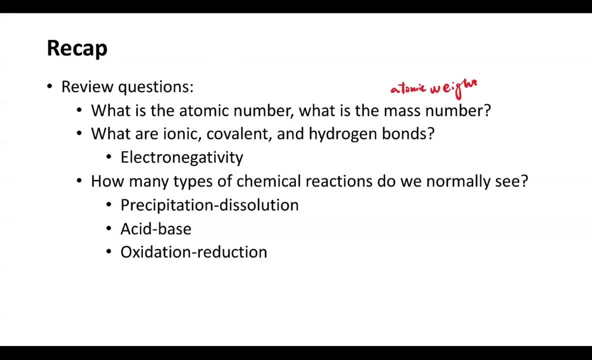 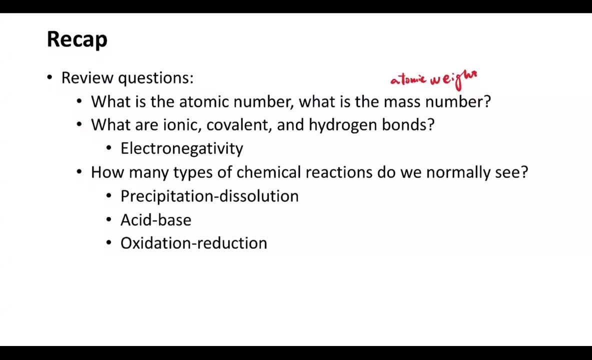 It's a situation where we consider the isotopes, because there are different distributions of the isotopes, So the average weight is going to have some digits after, or some have some digits after, the integer number there. So we also talk about what are the ionic and covalent bonds? right, It's mainly because of the different electron negativity of the elements. 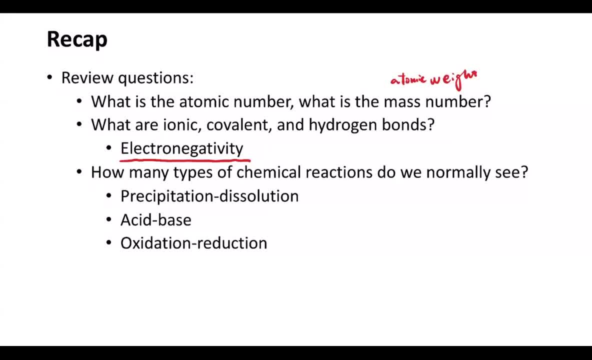 So we show the simple method to calculate Or to determine what bonds they should belong to. We can just calculate the difference of the electron negativity of the elements And then in that way we can calculate. So basically, if the difference is larger than 1.5 or larger or equal to 1.5, then the bond is ionic. If the difference is below 1.4 or equal to 1.4, the bond is covalent bond right. 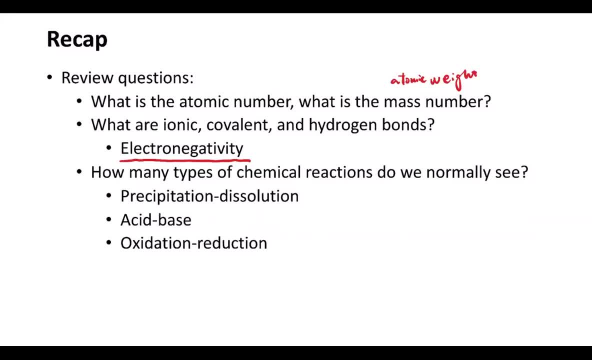 So we also generally introduced the typical types of bonds. So we also generally introduced the typical types of bonds. So for environmental engineering we're mainly going to learn about these reactions, right? So there are precipitation dissolution reaction, the acid-base reaction or the oxidation reduction reaction. 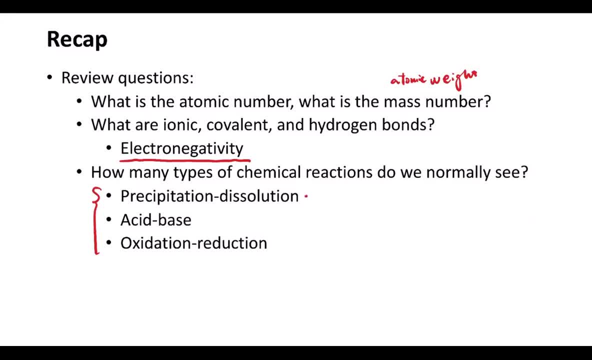 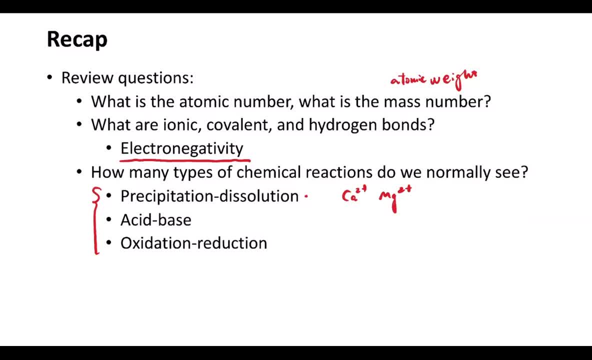 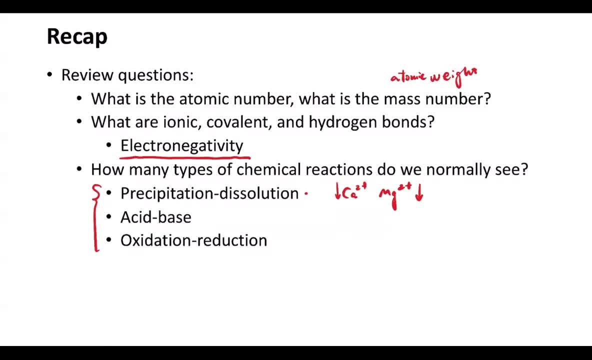 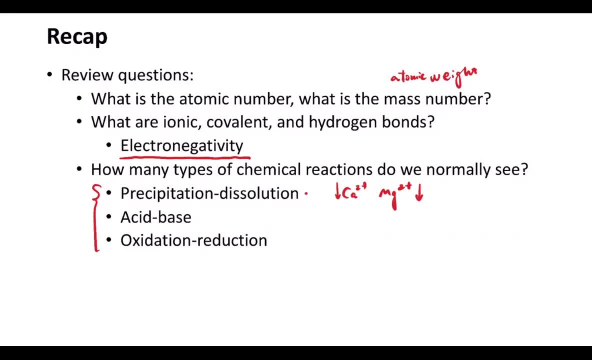 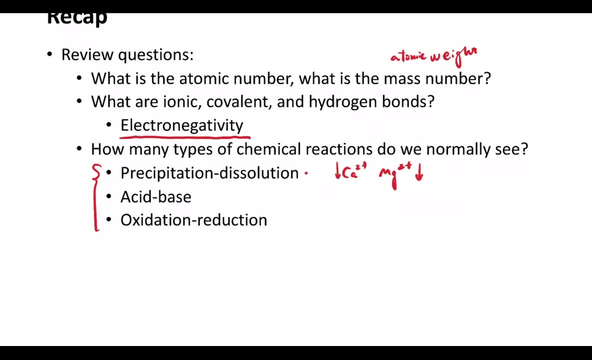 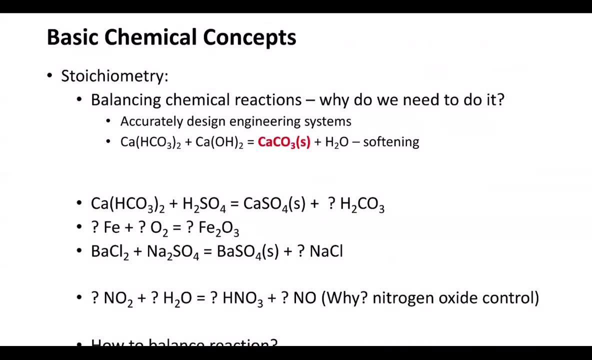 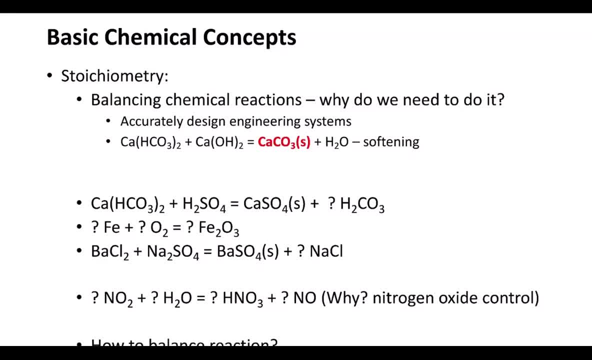 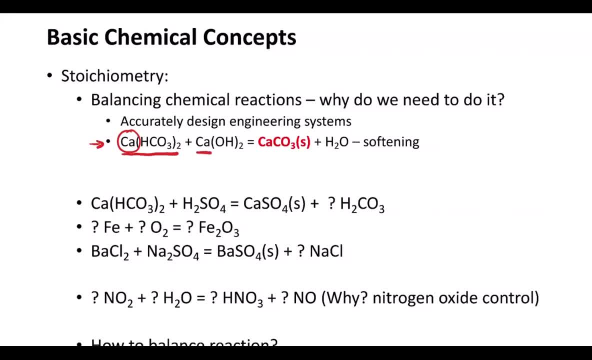 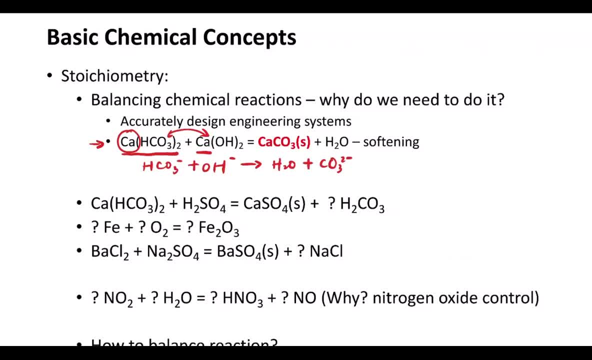 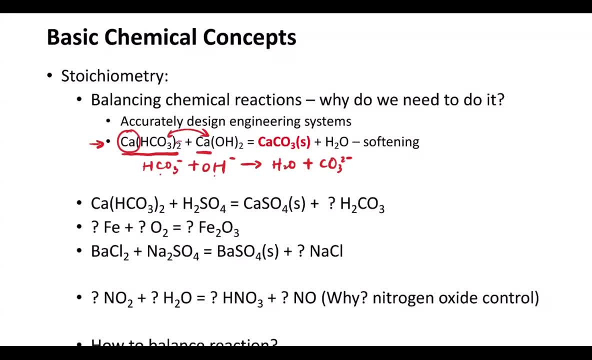 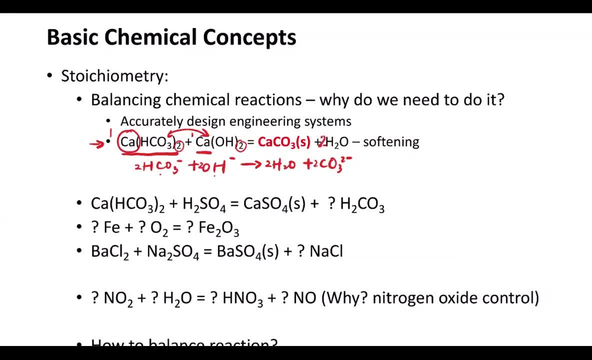 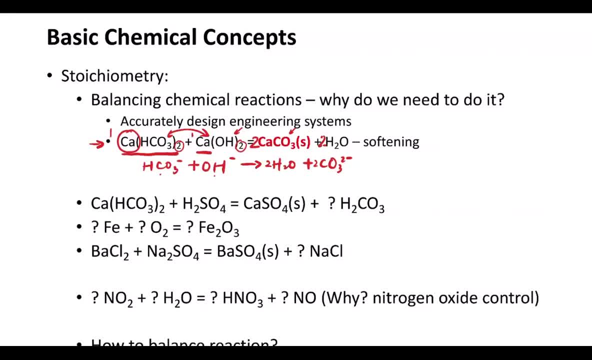 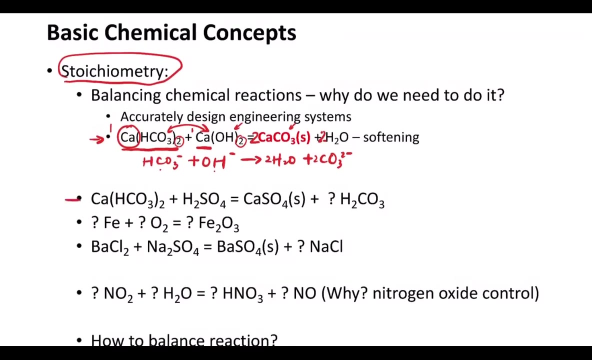 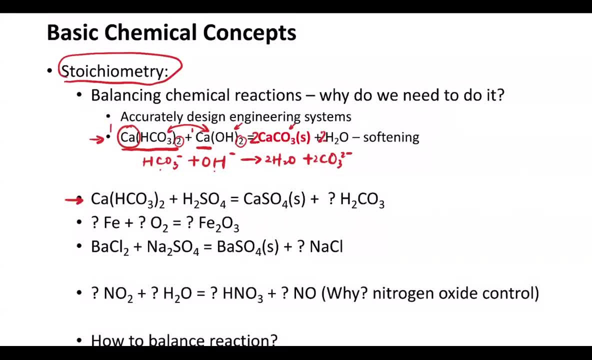 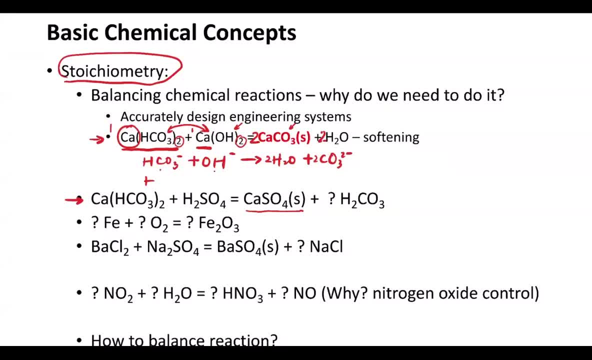 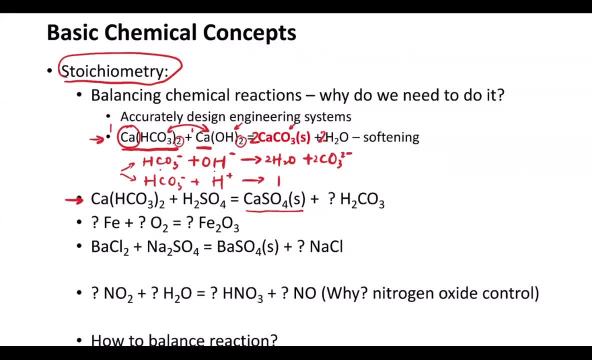 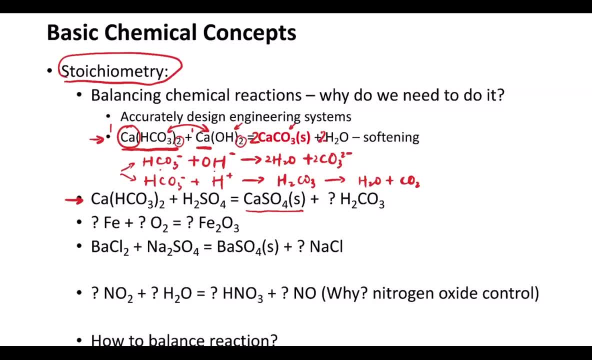 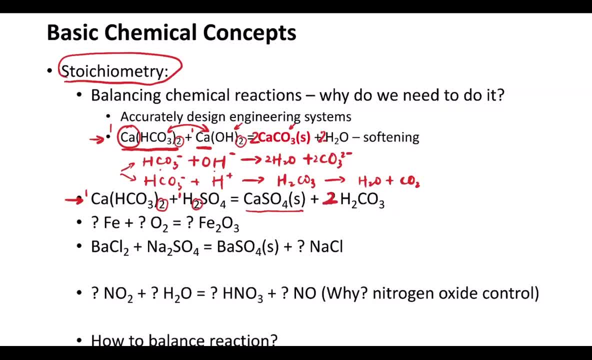 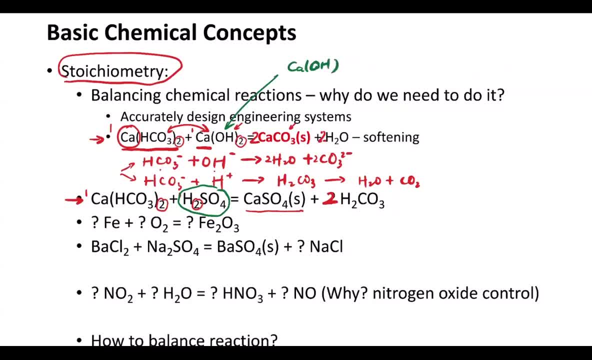 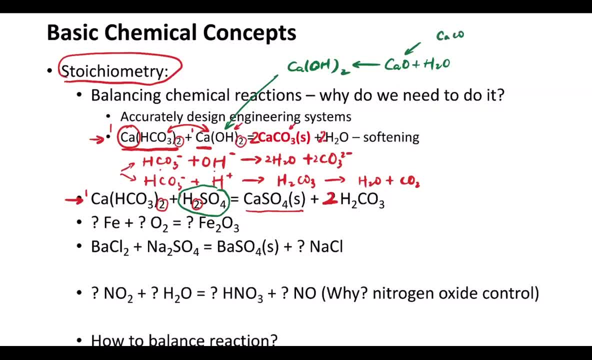 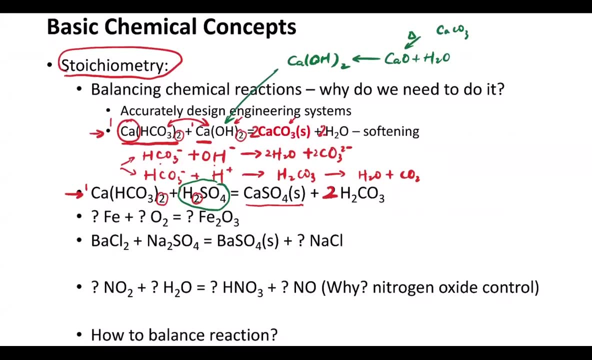 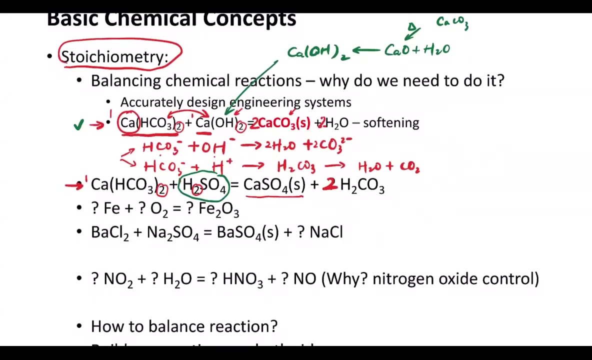 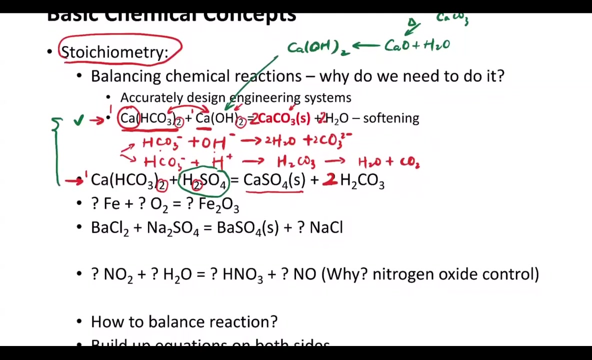 So for the precipitation dissolution reaction, we mentioned that a major application is the softening of the water, because the water has a lot of calcium ions and magnesium ions. So we also showed how to balance these equations. So basically, for these two equations we need to look at the ionic reactions. 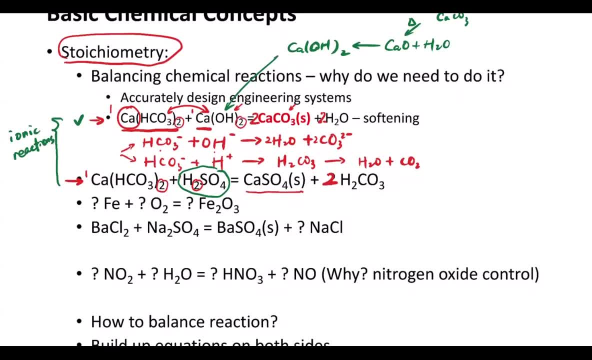 So the stoichiometry is determined by the stoichiometry for these ionic reactions. So here comes a simple one. So what about the iron getting oxidized into iron oxide? So we know that there are three number of oxygen elements on the right hand side. 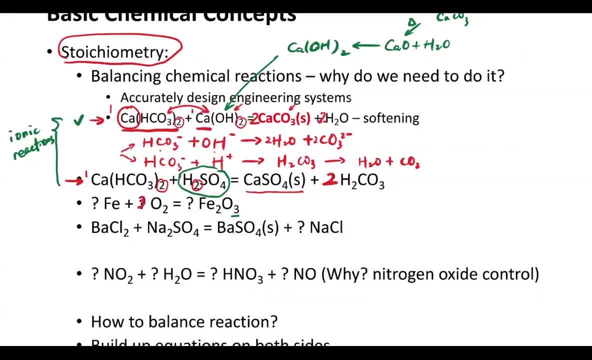 So the number in here should be three over two, over oxygen, And then we have two number of iron. So the number in front of the iron should be two. So if you want to rewrite this, then it's going to be four iron reacting with three oxygen. 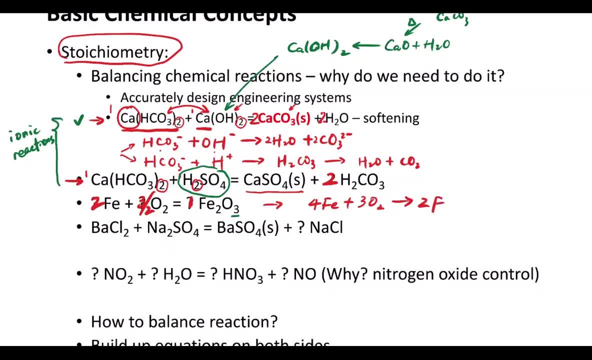 To form two iron oxide. So this is quite straightforward: You can directly count the number of atoms on the left hand side and right hand side to solve this balancing Right. So what about this reaction here? Barium chloride reacting with sodium sulfate Right. 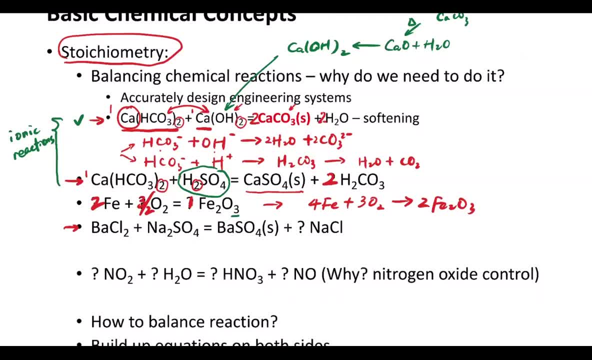 So this is quite similar to the ionic reactions that we talk about in the beginning, because we know that the barium ions can react, Can react with the sulfate ions and to form barium sulfate, which is a solid Right. So because these two ions are reacting at a one to one ratio, 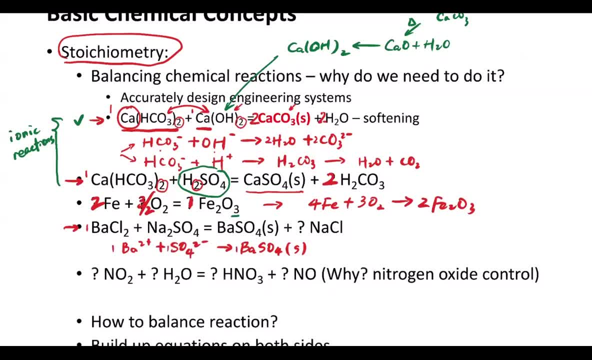 So these two compounds are going to react as a one to one ratio as well. Right, We're going to form one number of the barium sulfate, And then, by counting the sodium and chloride, We know that it's going to form two number of sodium chloride. 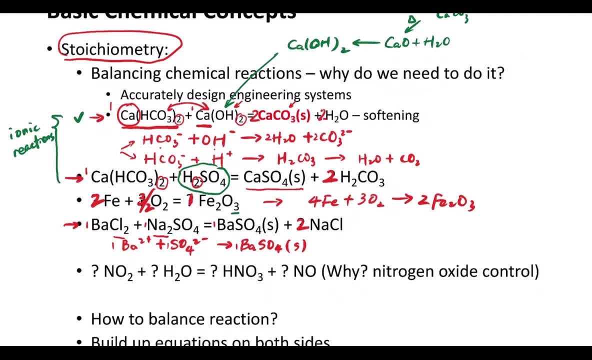 So this is how we can balance this reaction. So you can see that actually, I would say most of the equation balancing, or the reaction balancing, is quite straightforward As long as you know how the ions are reacting with each other. So what about this one? I guess that this reaction is a little bit challenging for us. 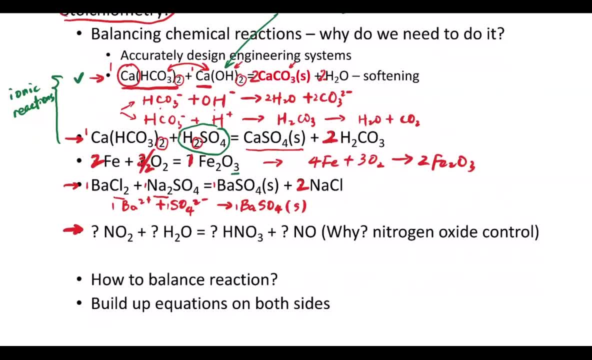 OK, so what happens is nitrogen dioxide is reacting with water to form Nitric acid and also nitrogen monoxide. OK, so why is it important? We can use this to control the nitrogen dioxide, which is a polluted gas species, So this reaction takes in the gas phase. OK, so this is actually the same reaction that's happening in the atmosphere. 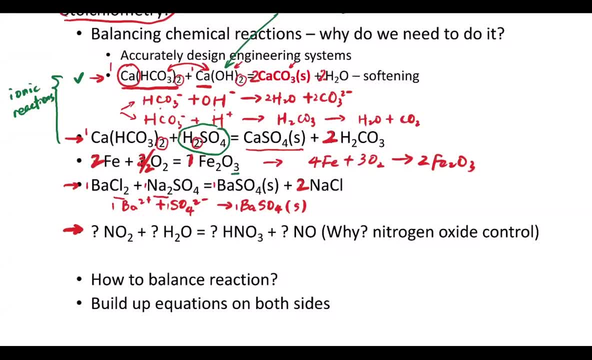 So always say something about the acid rain, Right? So if we emit the nitrogen dioxide into the atmosphere, they can react with water vapor and further form these nitric acid, So it's forming the acid rain. OK, so how to balance this reaction here? 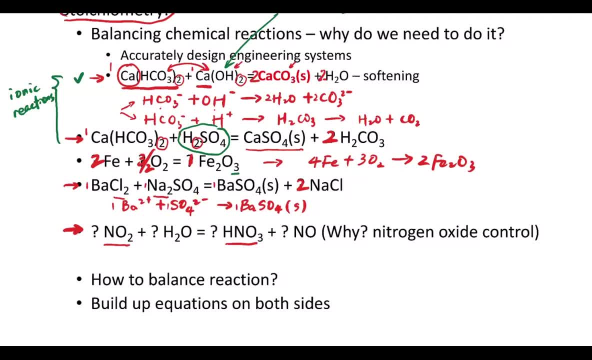 OK, so you see that it is a little bit complex because for a lot of the elements, let's say, there are just three elements here: hydrogen, oxygen and nitrogen. OK, so for oxygen and nitrogen they're showing up in almost all of all of the compounds, Right? 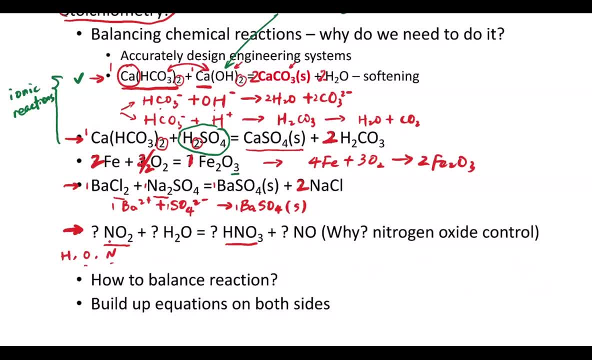 So, for example, nitrogen is showing up here, here and here, Oxygen is showing up in all of these compounds. OK, so we cannot assume that these two are reacting at a one to one ratio, because they can actually react in any ratio. 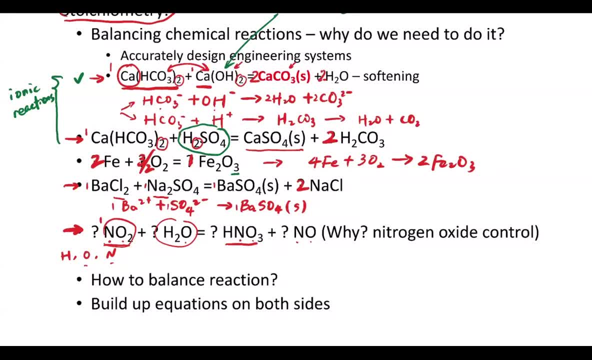 It can be. let's say, if we assume this to be one, this can be one, two, three, four, Anything, OK. so now, under this situation, we need to look for, We need to look for the unique elements, OK. 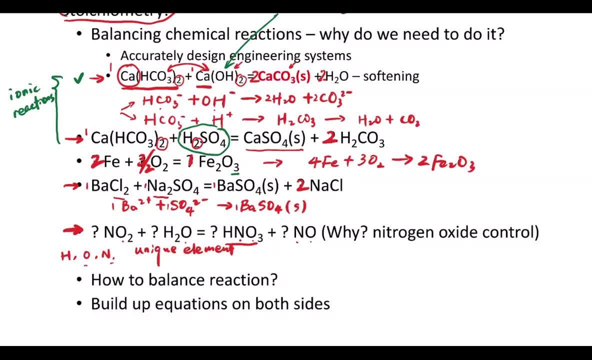 So the unique element is the element that just show up once on the left hand side and right hand side. OK, so you can see that we mentioned oxygen and nitrogen show up many times. So the unique element in this reaction is hydrogen. OK, so you see that the hydrogen just show up in the water on the left hand side and then in the nitric acid on the right hand side. 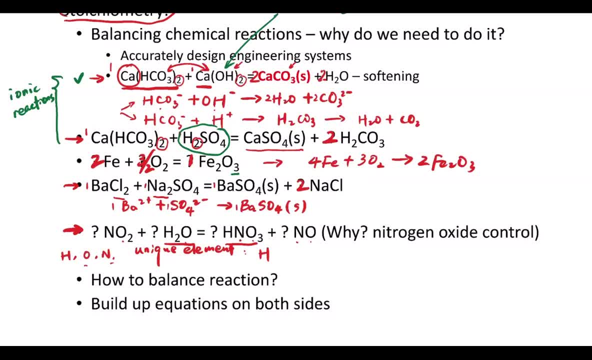 So now let's assume that the number in front of, in front of the water, is one, And then, because it just show up once, So the number in front of the nitric acid is two. OK, so now we don't know these two numbers. We can assume that to be then to be, X and Y here. 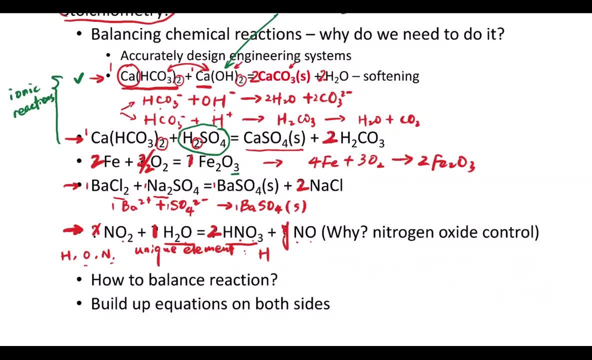 And we can basically set up a equation. OK, so we have two unknowns and two equations, each for the oxygen and nitrogen. All right. So for oxygen, to set up this balance, it's going to be to multiply by X Plus one Right. That's for the water. And on the right hand side, 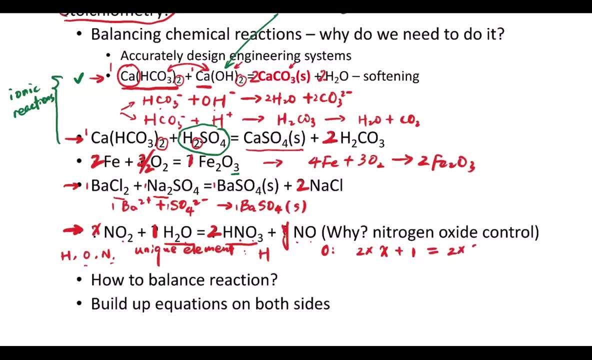 And on the right hand side, that's going to be to multiply by, multiply by three Plus Why? OK, so for nitrogen, that's going to be to multiply by X, Equal to Two plus Y. OK, So if we just simplify these equations, 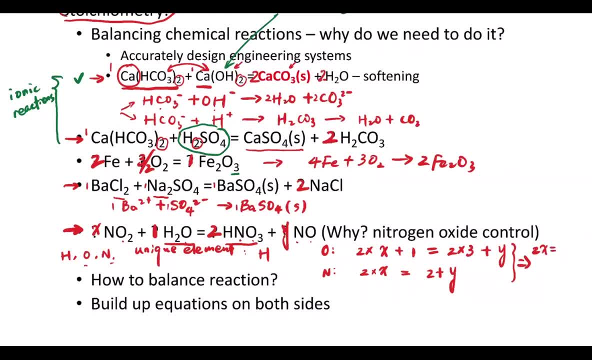 A little bit. So that's two X Equal to five plus Y, And two X equal to See OK. so I think I made a mistake here. So for nitrogen, OK. so for nitrogen. here It should just be X. 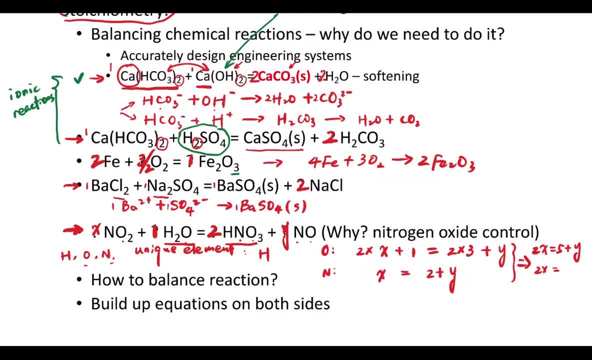 OK, so on the left hand side for nitrogen that's a single single nitrogen atom Right. So that should be X equal to two plus Y. So if we just use this equation to minus The second equation, we have X equal to three Right. 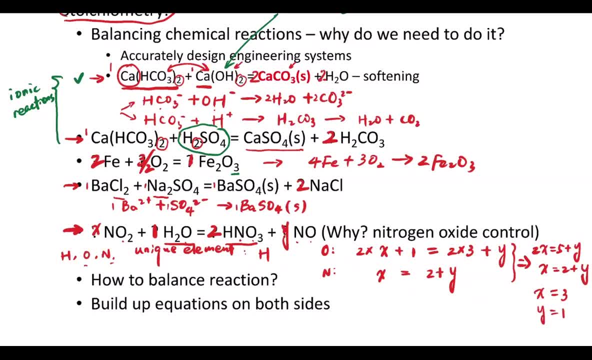 And then if X equal to three, then Y is equal to one If we plug in this number here. So basically, by setting up these equations we can further solve what is a number in front of these chemical compounds? Right, So now we know the X and Y are going to be three in here and one in here. 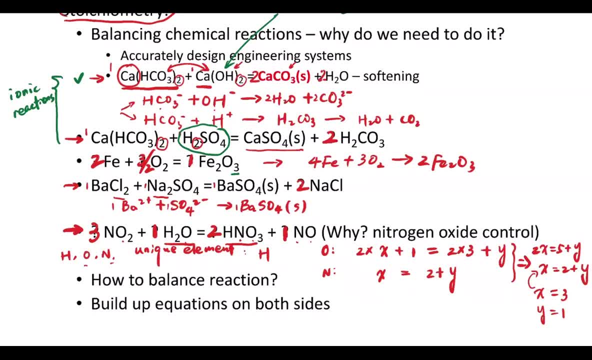 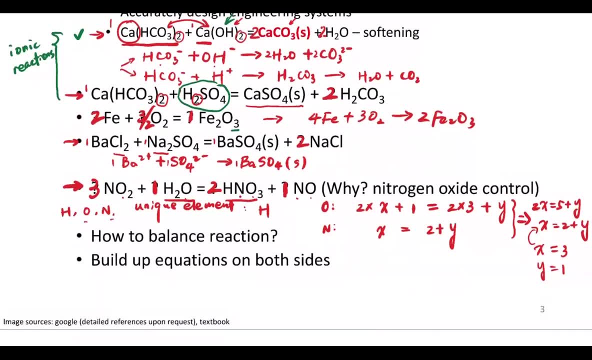 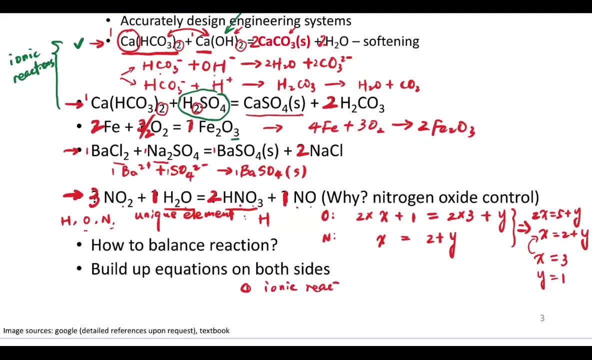 OK, so this is how we approach a little bit more complex chemical reactions. So now, if we summarize how to balance the equation, OK, so for the simple ones, we should rely on the ionic reactions. So based on the stoichiometry of these ions, 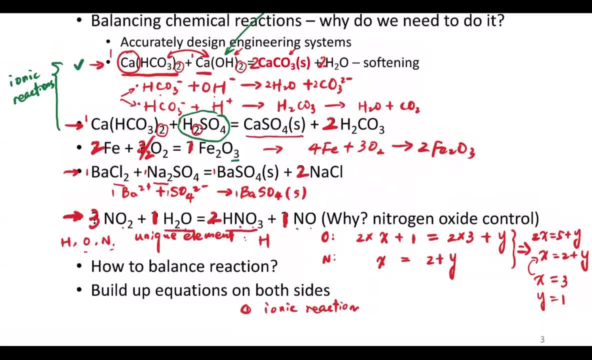 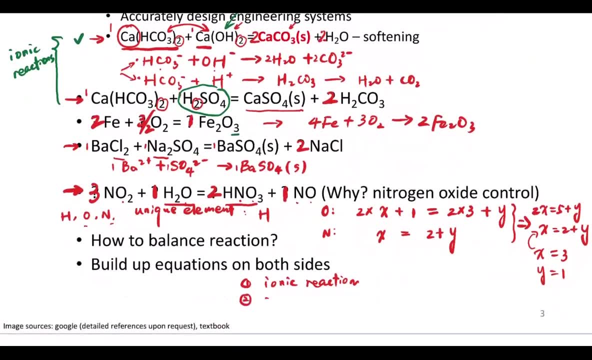 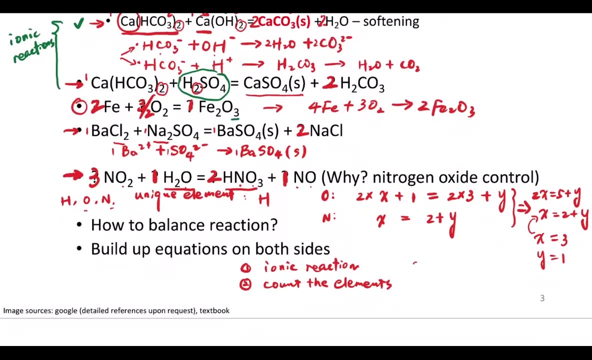 Right, We can calculate. We can calculate what is the stoichiometry for the compounds, Or we can directly count. Count the elements, So similar to this one, All right. So for a little bit complex ones, then we need to first. 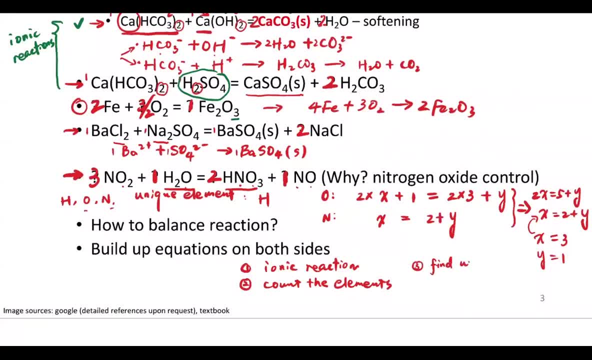 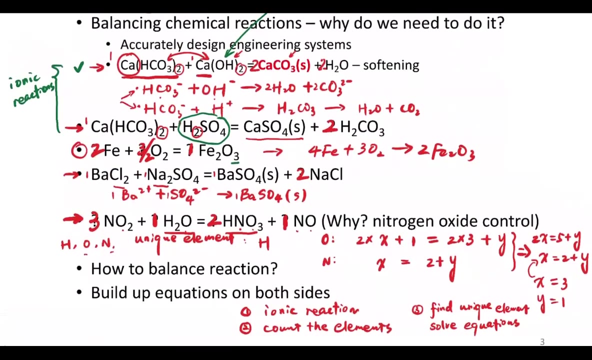 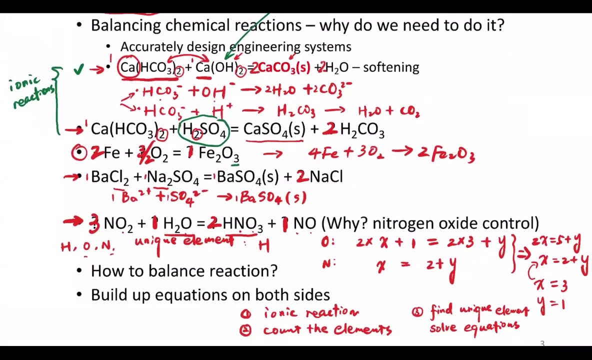 Find the unique element And then we should set up equations Right Or to solve Equations. OK, so this is how we can balance the equation Right And, as we said, they have very important engineering applications. So later in this class we can find out basically how we use the balance, the equations, to calculate or to design these water treatment or air pollution control device. 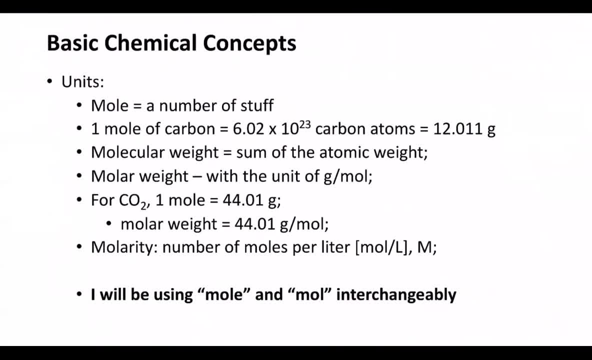 Right, So that is something quite simple. So I'm pretty sure that All of you guys know What a mole means. So a mole means a number of stuff. OK, so let's say, if we mention a mole of carbon, it means 6.02 multiplied by 10 to the 23rd of the carbon atoms. 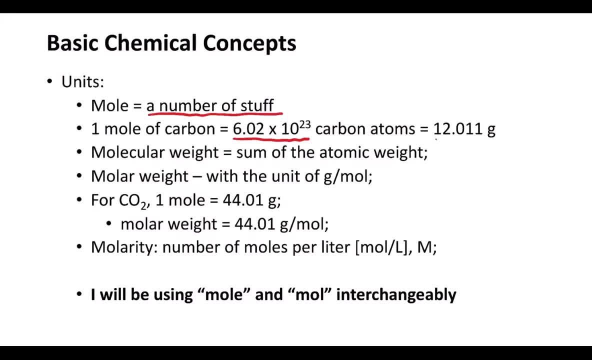 So that turns out to have a have a mass of 12.011 grams. OK, So we mentioned why this number has quite a lot of digits after it, After the integer Right, Because of the isotopes Right. So this is associated with the atomic weight. 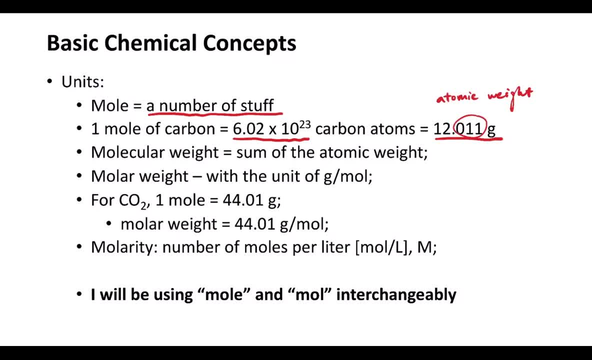 So last class we mentioned, we also mentioned that there is a similar definition for the molecules, Right. So the molecular weight. Molecular weight means that we just need to sum up all the atomic weight. So we showed that for the calcium carbonate. So it's a value of around one point, one hundred point zero eight. 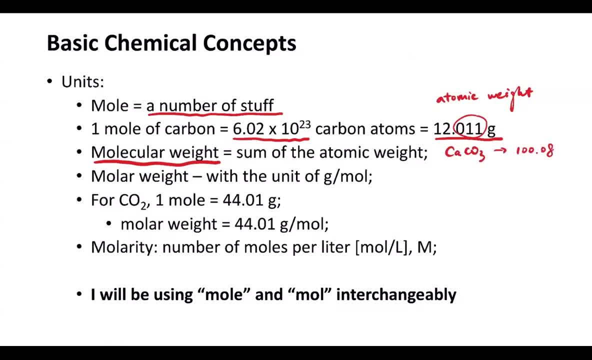 Right, So based on the molecular weight people also define the molar weight. So basically, the molar weight means the weight per mole of stuff. OK, So it has the unit of gram per mole, Right? So for example, for carbon dioxide it has the molar weight of 44.01 gram per mole. 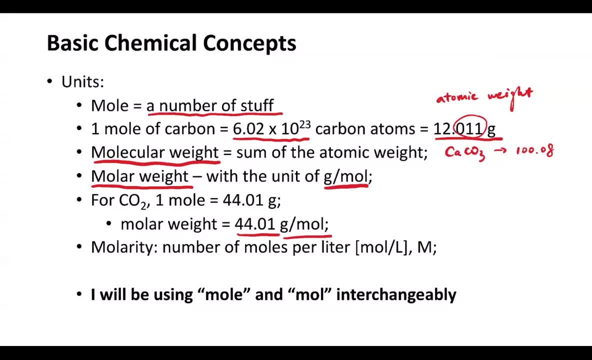 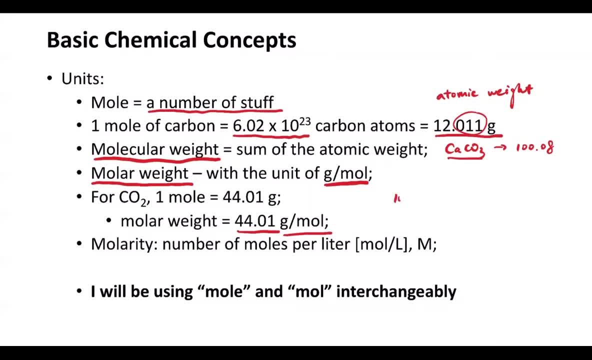 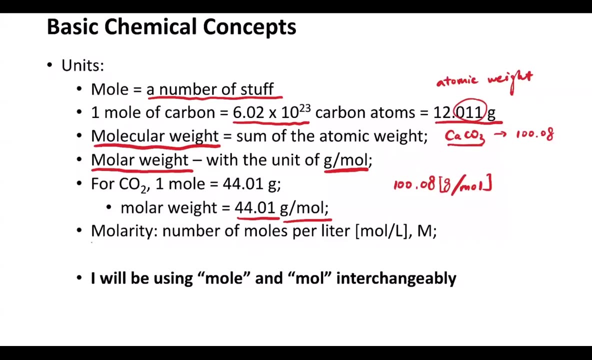 And similarly for the calcium carbonate, it has the molar weight of one hundred point zero eight gram per mole. OK, So this is a molar weight. So in water treatment and treatment and wastewater treatment there are also a term called the molarity. 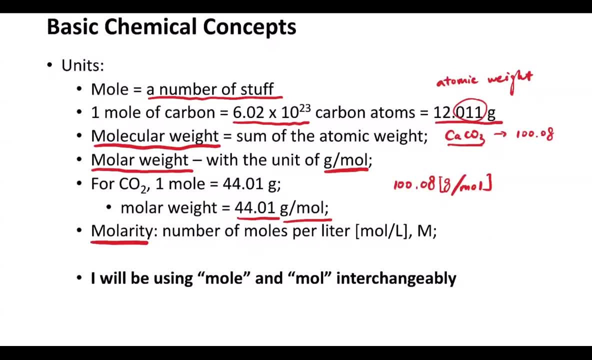 OK, So the molarity basically means the concentration of some substance, The concentration of some species in water. OK, So it means the number of moles per liter. OK, So, generally it has the unit of mole per liter. And then, more specifically, when people use the term molarity, then the unit is going to be 1m. 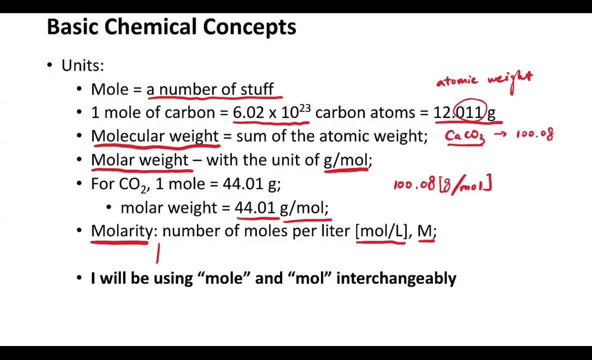 So let's say, for example, we have a bottle of water. OK, So the bottle of water has some sodium chloride being dissolved If we say the molarity of the sodium chloride. let's say molarity of sodium chloride is 1m. 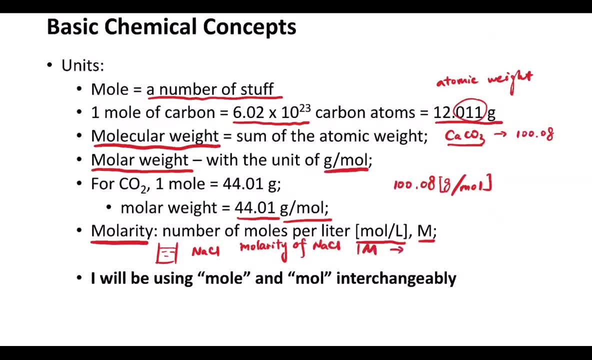 It simply means that the concentration of the sodium chloride in the water is one mole per liter. OK, So this is what the 1m means, But for a lot of the water systems we're not dealing with a very high concentration of these compounds. 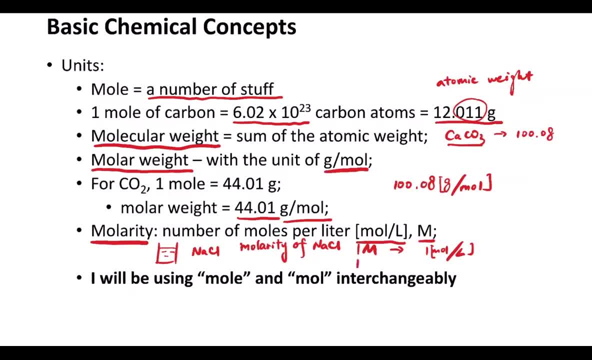 So that's why people also design the unit of 1m. OK, So that's just one thousandth of this concentration here. So what that means is one millimole per liter, Or you can think of it as 0.001 mole per liter. 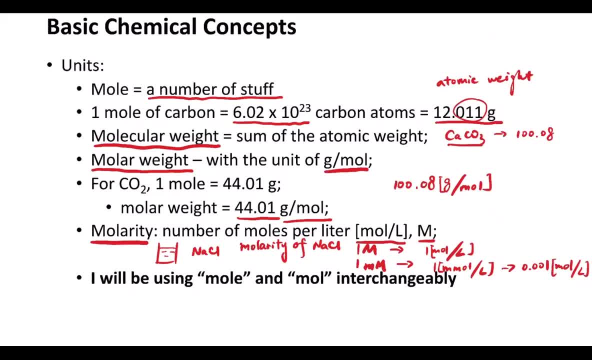 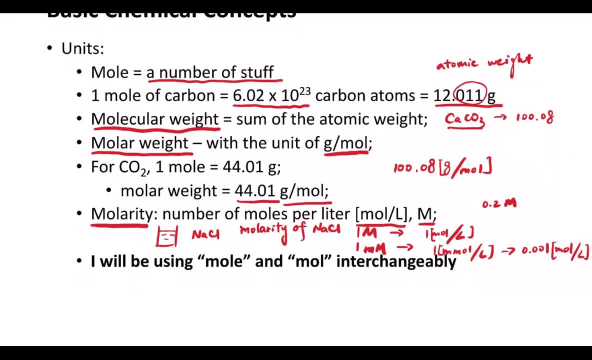 OK, So this is what the molarity means. So in the future, if you see the concentration of certain species in water, Let's say it's 0.2m. So that simply means the concentration is 0.2 mole per liter. 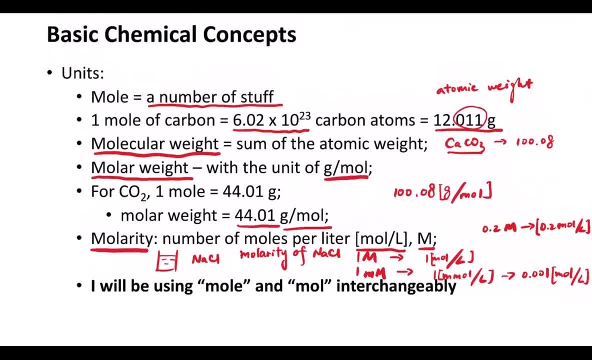 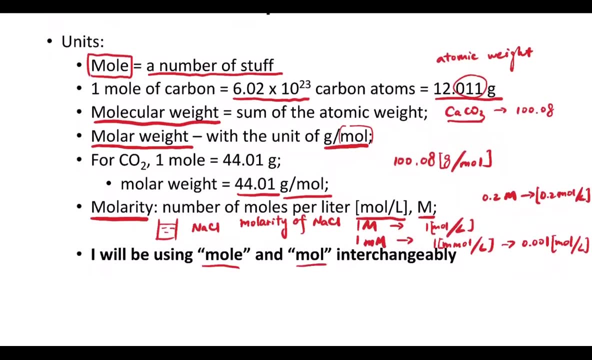 OK. So, as you can see from this slide, I use the mole in the foo term or in the foo name, And sometimes I use the mole in, let's say, just the three letters. So in this class I'll be using this foo name and this type of mole interchangeably. 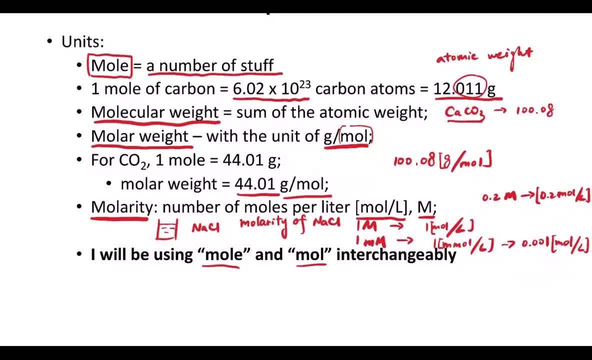 So basically they mean the same thing. I know that in the textbook, probably when they describe the mole, they're going to use the entire name, But when they are shown in the units we're just going to show the three, the first three letters here. 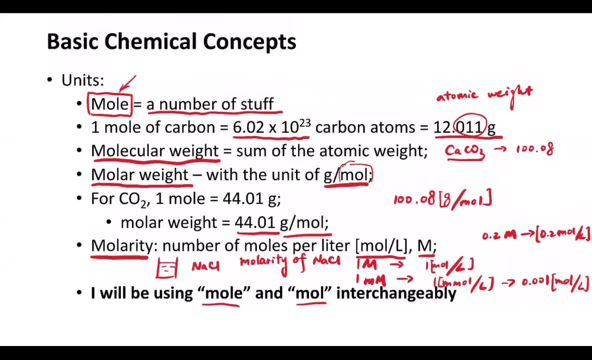 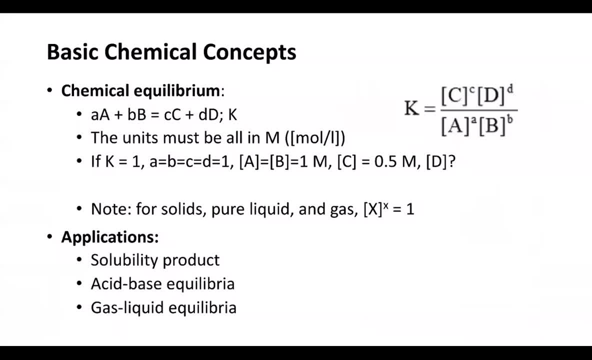 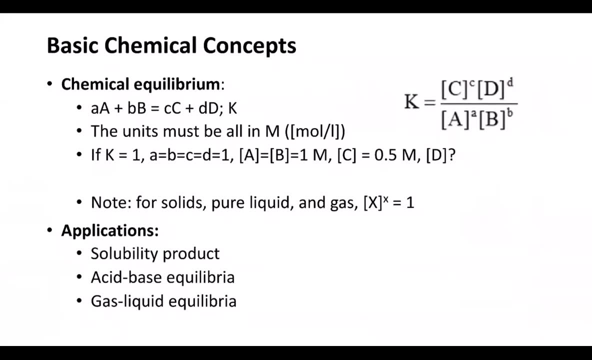 OK, So this is about the moles, the concentration and the molarity. So now here is something a little bit complex. OK, So this is the chemical equilibrium. I hope that most of you know what this means, But if you forgot, so basically chemical equilibrium means the final state, or determines the final state of a reaction. 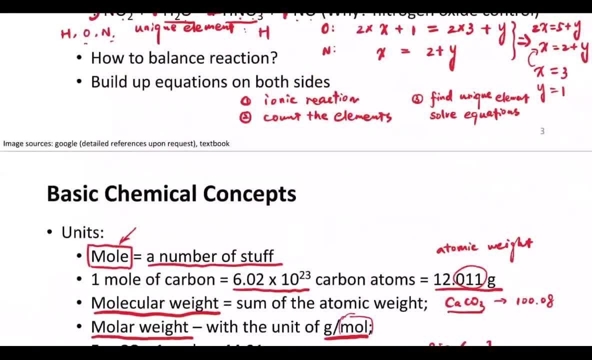 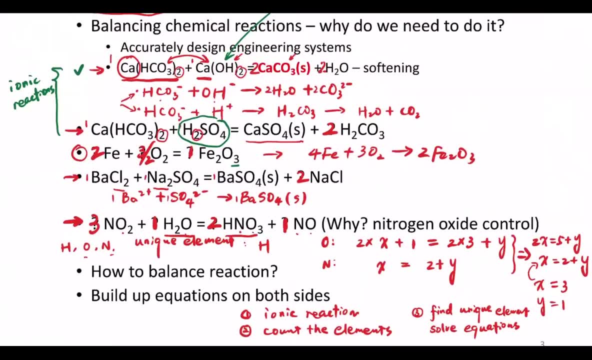 So, for example, if we go back to these reactions that we talked about earlier, So although we write out these reactions with the symbol of the equate or the equation symbol, the equation symbol doesn't mean that this reaction will happen completely. It doesn't mean that, let's say, if we have one mole of calcium, let's say one mole of the calcium bicarbonate. 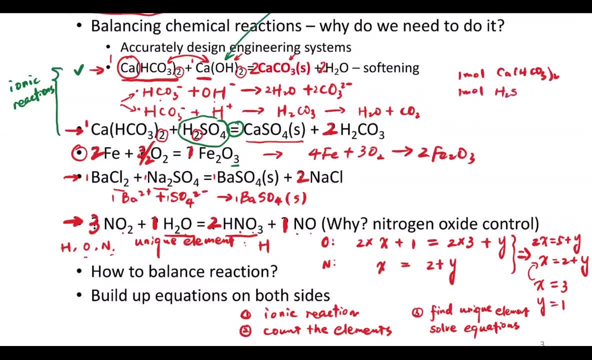 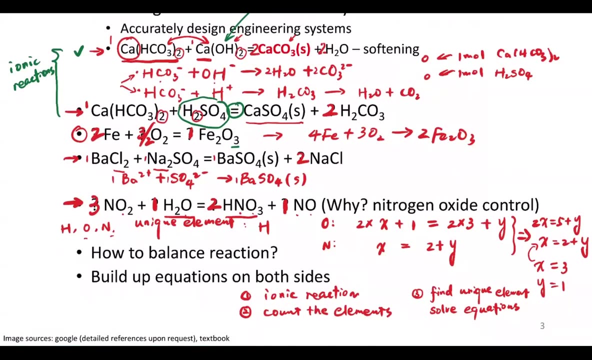 And one mole of the sulfuric acid, It doesn't mean that these two will react completely and get into zero. OK, So for all the reactions There's basically There's none of the reactions that can happen completely, So there is always a final state that both the reactants and the products coexist. 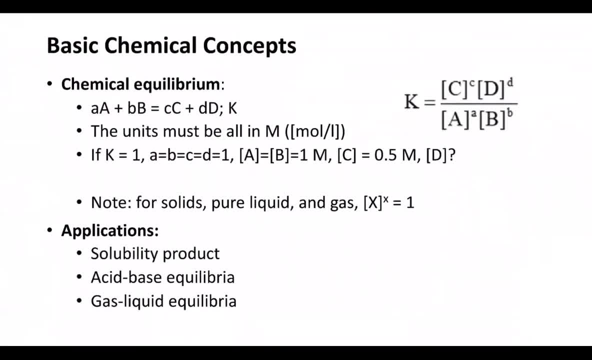 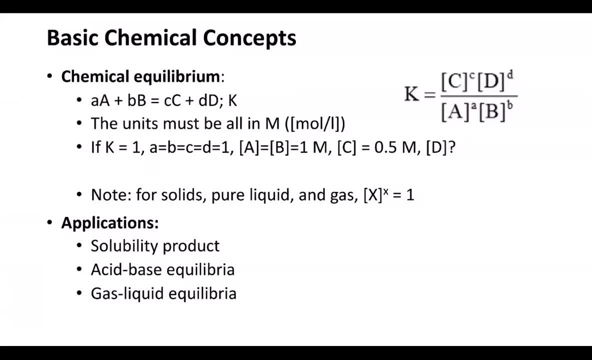 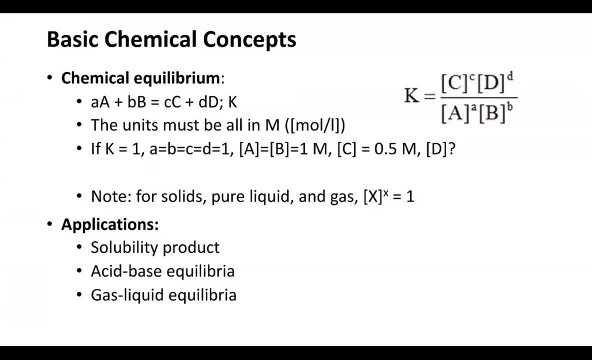 So we're talking about the final state basically taking a very long time. It can be months or days, months, years or thousands of years. OK, so we're talking about that final state, All right. So the chemical equilibrium determines what the final state look like. 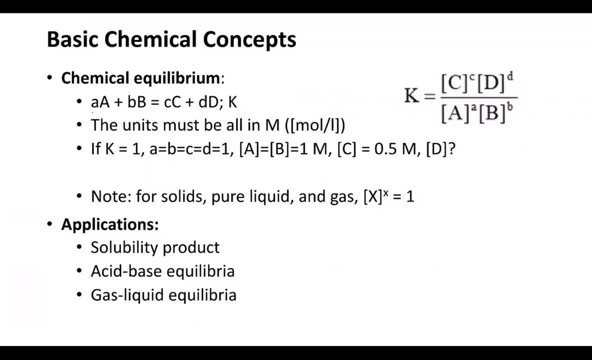 OK. So, for example, if you have this reaction here, So A number of A reacting with B, number of B to form C, number of C and D, number of D. OK, So what people? the way people define this final state is by creating a number that's called the equilibrium constant. 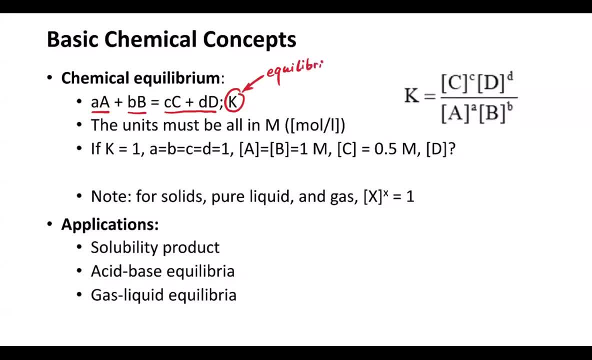 OK, So the equilibrium constant is calculated by the concentration of C to the power of C, And then multiply the concentration of D to the power of D. Divide by the concentration of A to the power of A. Multiply the concentration of B to the power of B. 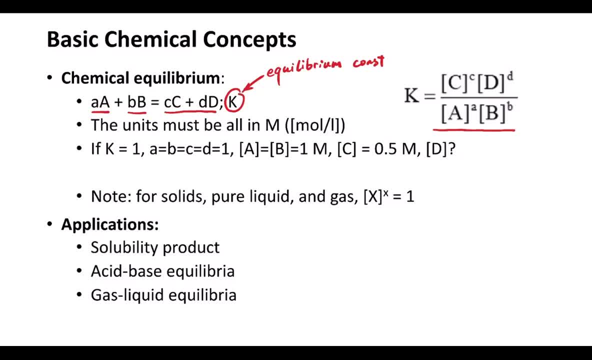 OK, So basically, it's the product to certain power for the product of the reaction Divide by the product regarding the reactance of this reaction. OK, So the equilibrium constant, as it says, is always a constant. It may be dependent on the temperature. 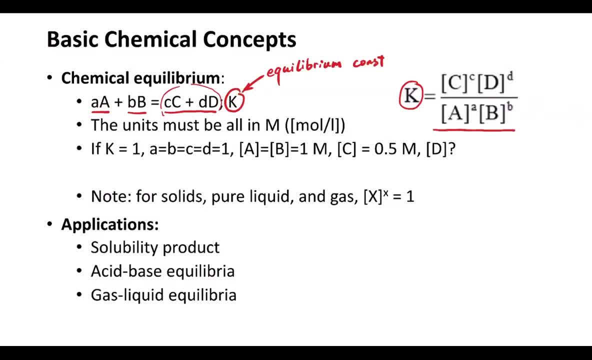 Actually it is dependent on the temperature, But at certain temperature this is always a constant, OK. So one thing we need to notice is that all of these must be shown in the unit of M, So recall that for molarity we have this unit here. 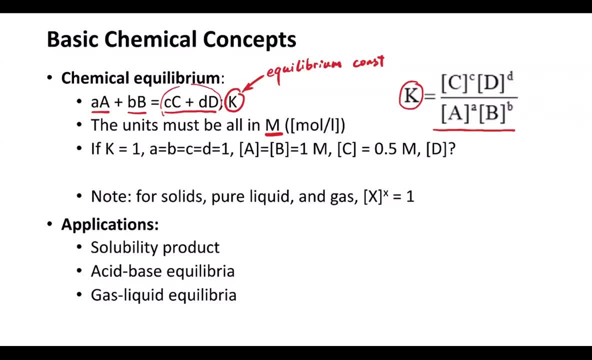 M right, It basically means mole per liter. OK, So just to do a quick practice. So let's say that if we have a reaction that has all of these coefficients to be one, So basically it's A plus B going to C plus D. 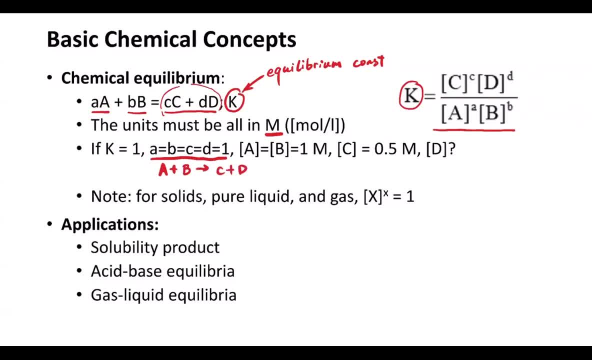 OK, So for this reaction, if we know that, let's say, under 25 Celsius the K is equal to one, So further we have the concentration of A and B and the concentration of C. So what is the concentration of D? 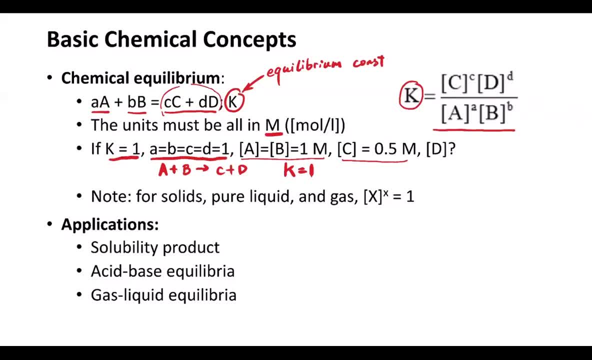 So let's do a quick pooling on this problem here. I think it should be quite straightforward, OK. So let's give it 10 more seconds, OK, All right, We'll stop here, OK, So I will share the results. 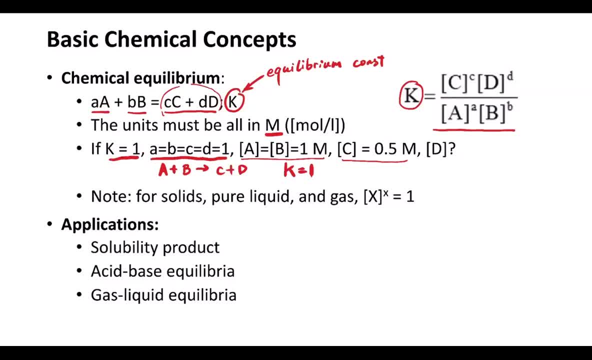 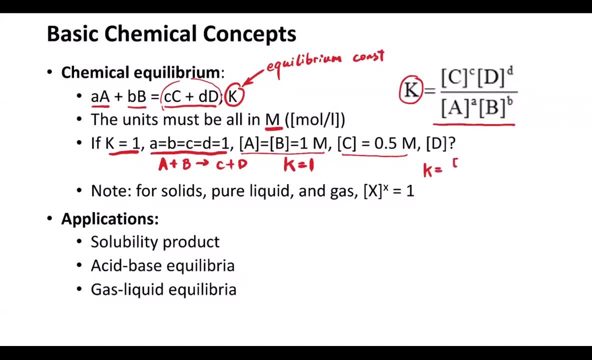 So most of you guys are correct, So it should be 2M, OK. So if we set up this equilibrium constant, we know that K is equal to C to the power of one multiplied by D, to the power of one divided by A, to the power of one multiplied by B to the power of one. 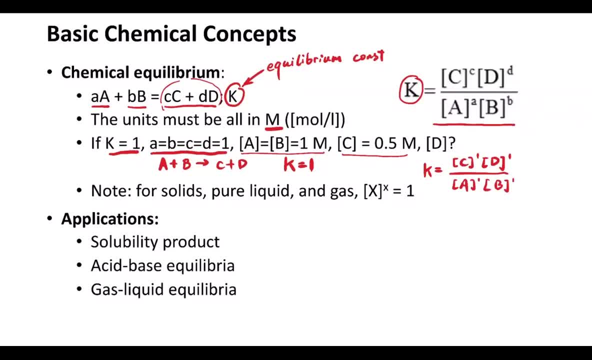 Mainly because the lower case, A, B and C and D, are all equal to one Right. So because of that, this term is equal to one. OK, So further we know the concentration of A and B. These are one one. 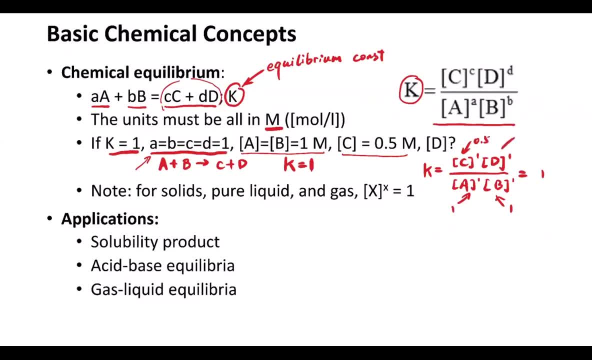 So C is equal to 0.5.. So because of that, D should be equal to 2M. OK, So basically what this means is that for this reaction, although we're using this equate sign here, it doesn't mean that this reaction will be equal to 0.5.. 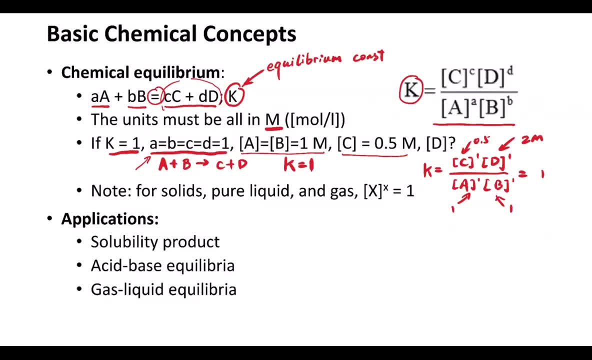 OK, reaction will happen completely. Actually, none of the reactions are going to happen completely, Right? So there's always some reactants and some products coexisting in the system. OK, so I also want to put a note here. So for this equilibrium, constant here, that's. 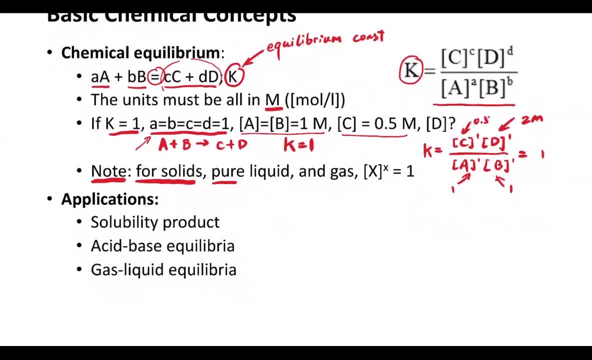 defined here for solids or pure liquid or gas. So if they happen to show up in this reaction here, then their term- basically it's the concentration to the power of X- should be always equal to one. So we're referring to basically the formation of solids, Right? 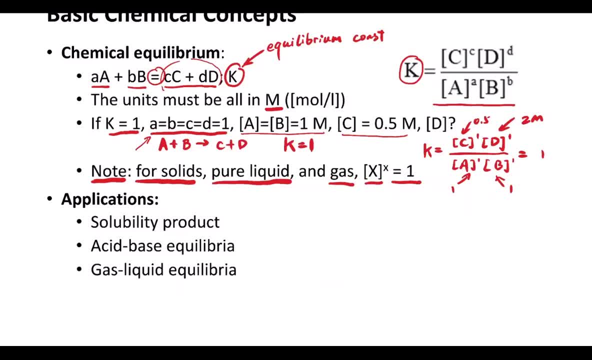 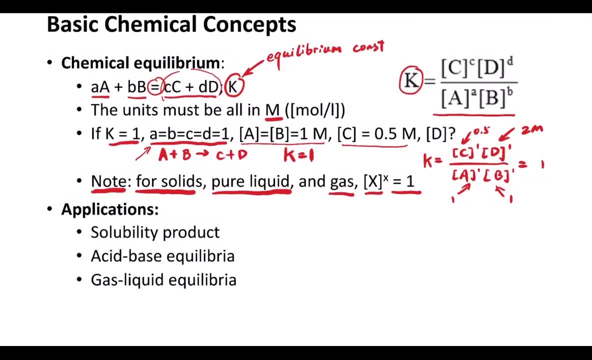 So, if you recall, for the water softening Right, So there are some solids being formed in that reaction there. So if that's the case, then we don't need to consider the concentration of the solid or we don't need to consider the concentration of the pure liquid. 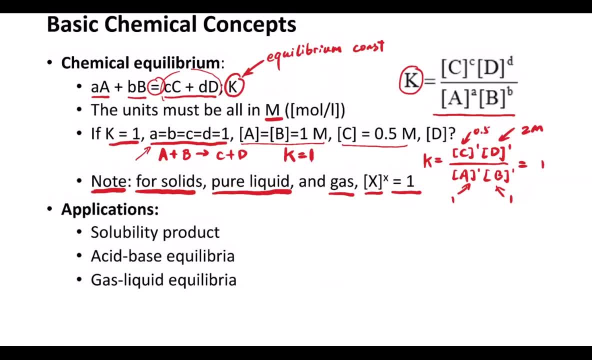 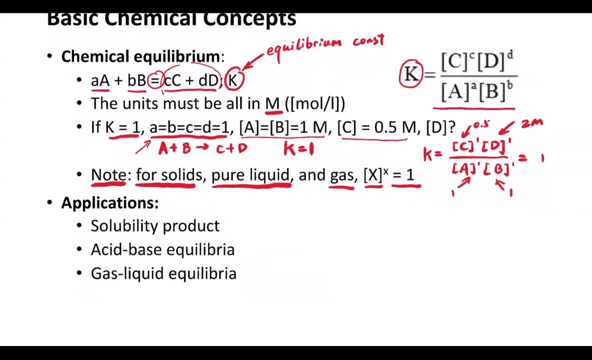 OK, so we're going to give some examples in the in the next few slides. So what is the application of the chemical equilibrium? So there are three major applications in environmental engineering. So one is a solubility product, One is the acid. 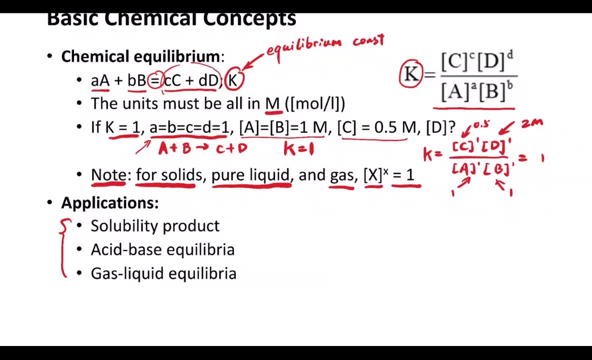 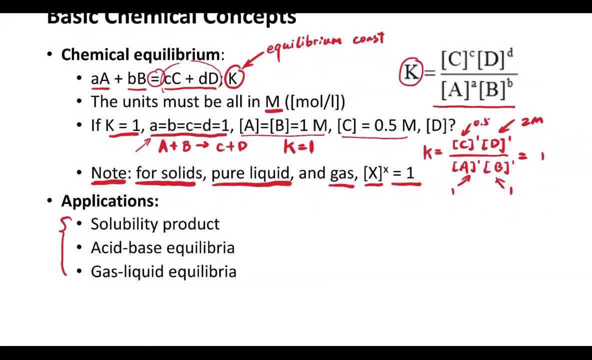 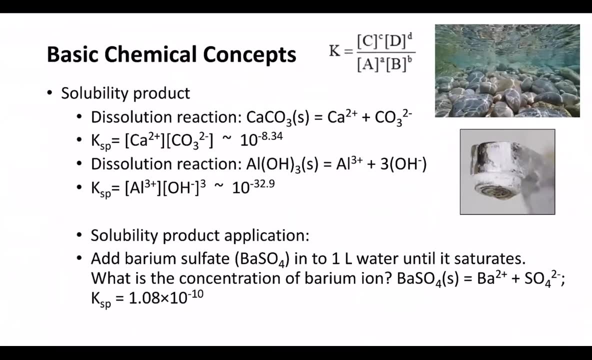 base equilibrium or equilibria. And one is the gas liquid equilibrium, equilibrium. OK, so first about the solubility product. So the solubility product means Basically any solid are going to dissolve some part of the solid into the water. 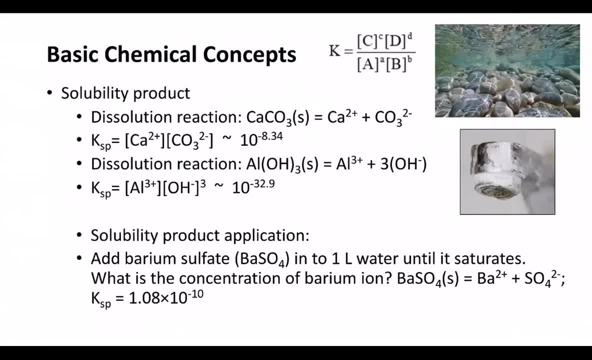 So? so you may wonder. well, the rocks are rocks, right? There is no way that they can dissolve in water. So why do we care about this, This dissolution here? So, actually, when we talk about the water hardness, right, the white scale, 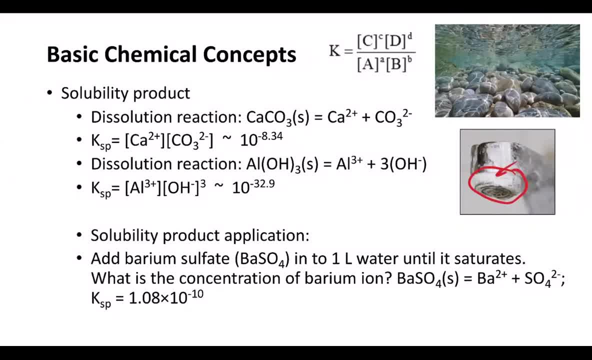 that's forming on the faucet, as we mentioned, it's because of the calcium ions, And actually these calcium ions are coming from these rocks. OK, so they are always some part of the solid that can dissolve into the water. Although this 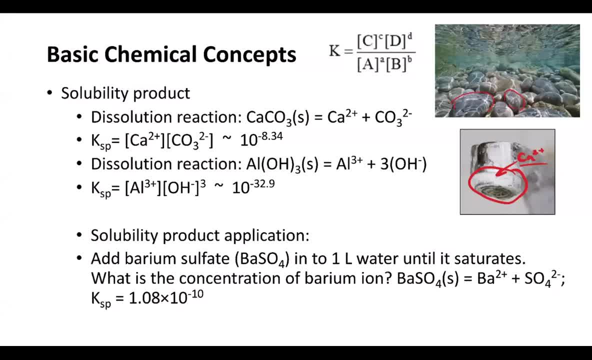 dissolution is just happening for a little bit. it's not completely dissolved, Right, So there's a small fraction of the solid That can get dissolved into the water. OK, so, for example, if we're talking about the dissolution of the calcium, 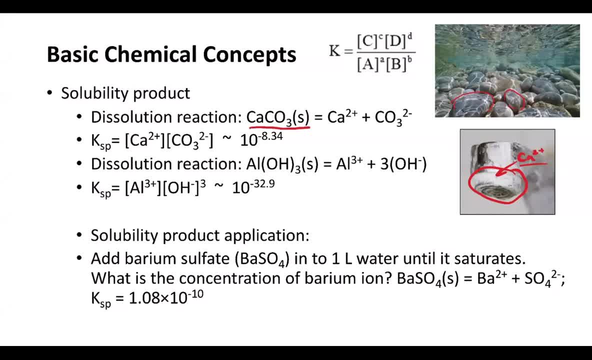 carbonate. so we know that this is basically the limestone. If we, if you dissolve or if you just directly emerge this limestone into water, there are some dissolution. OK, so how to determine the concentration of the ions? OK, so we're going. 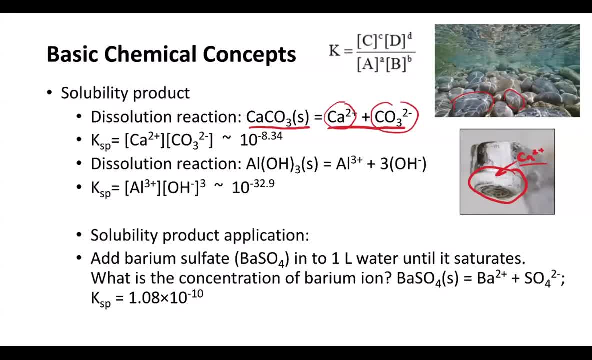 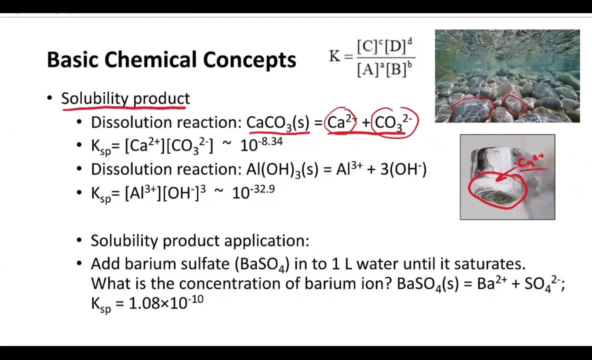 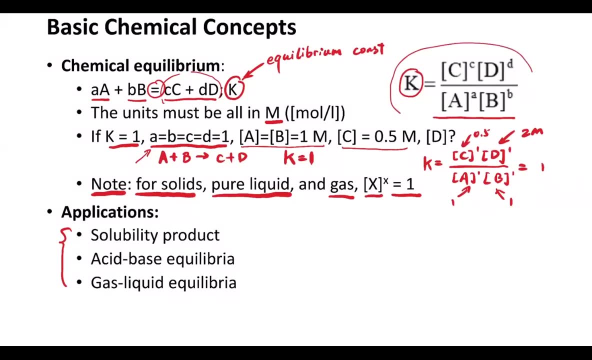 to use this chemical equilibrium or, more specifically, we're going to use the concept of the solubility product. OK, so, if you recall, for any reaction, right, so for any reaction, the equilibrium constant is written in this way. So similarly we can write out the equilibrium: 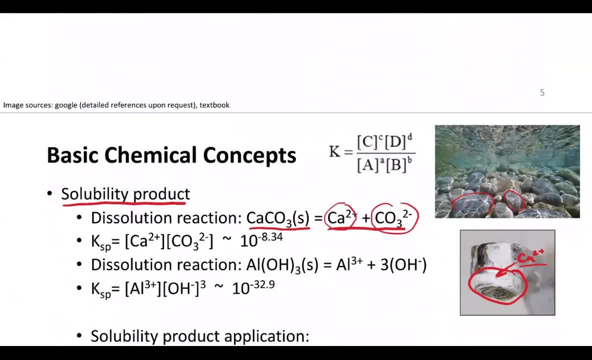 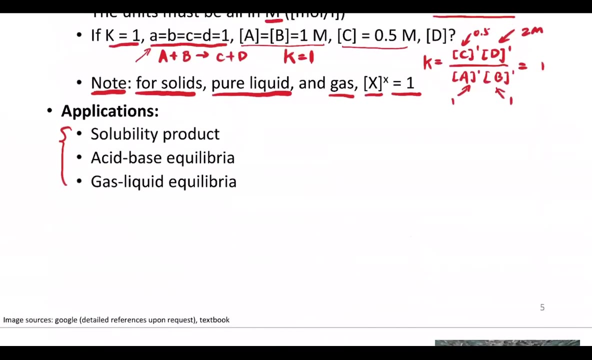 constant for this reaction. So that's going to be the concentration of the calcium ions multiplied by the concentration of the carbonate ions, Divide by the concentration of the calcium carbonate. OK, so all of them are to the power of one. So further, if you follow the note. 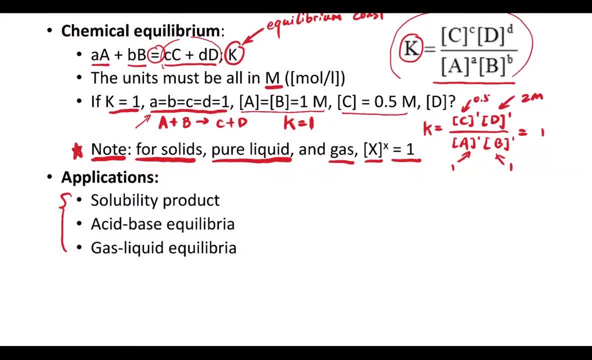 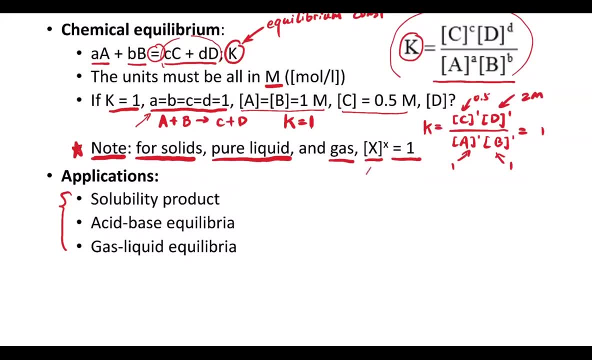 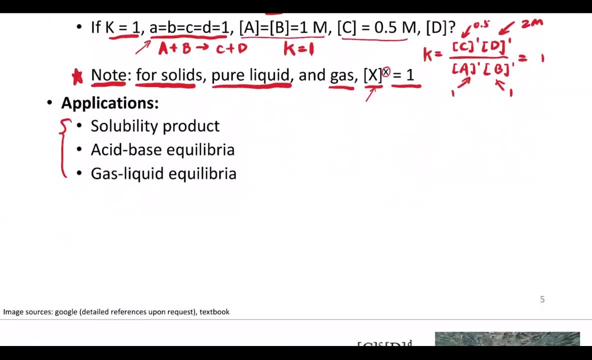 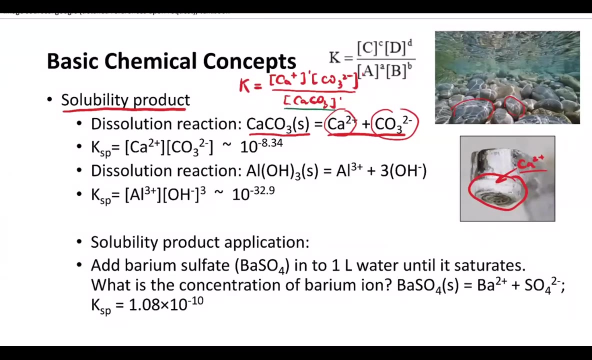 that we mentioned here. So for solids, pure liquid and gas, their terms should be equal to one. So basically the concentration of this solid to the power of the coefficient should be equal to one. So if we apply that into this dissolution here, then this term in the denominator should: 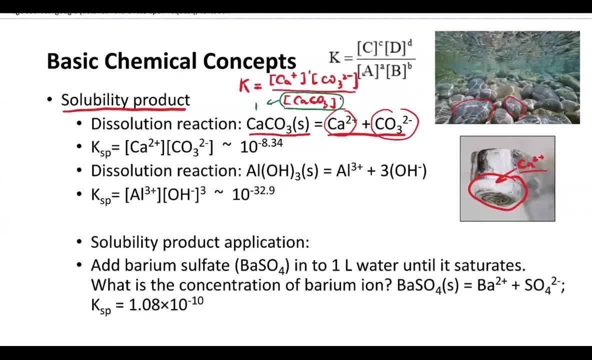 be one, Right? So basically, for this reaction here, or the dissolution of the solid, then the equilibrium constant is just a product of the. basically, it's a product of the products that's coming out of this reaction here, Right? So, more specifically, we're going to add a subscript. 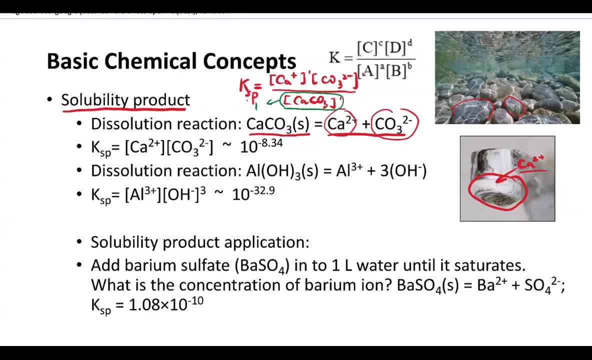 sp here to show that it means solubility product. OK, so basically for this reaction here people have measured or determined what is the equilibrium constant, or the solubility product or the KSP? OK, so it turns out that for this reaction the KSP has a value of around 10 to the negative. 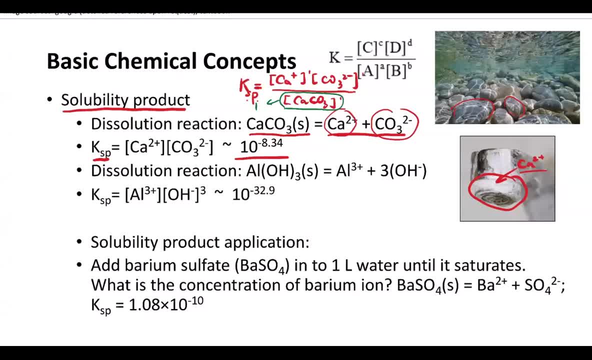 8.3. 4. OK, so this is a very small value, Right? So what that means is that, so the product of these two concentrations should be equal to this value, Right? And then you can find out how small this is. So let's assume further. assume that these two concentrations are: 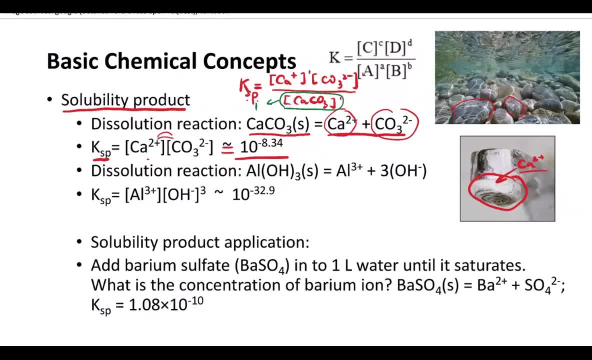 equal to each other because they are dissolving at a one to one ratio. Right, So what you have is the calcium ion to the power of two is equal to 10, to the negative eight point three, four. So further, the calcium ions concentration is equal to the square root of 10 to negative eight point three, four. 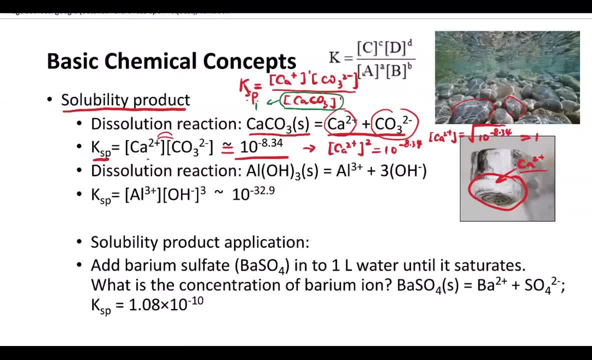 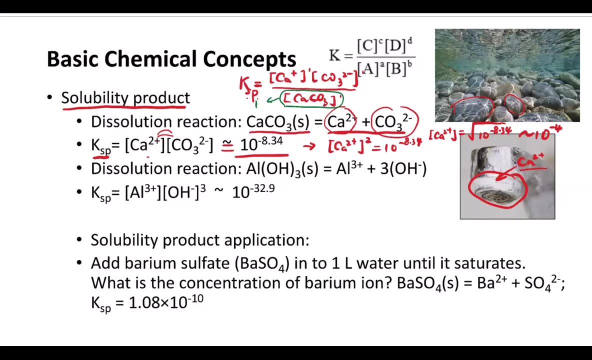 OK, so this turns out to be around, Let's say, Let's say around 10 to the negative four. So this is a very small, very low concentration, Right? So that's why these Solids, they're not dissolving a large fraction of them, Right? It's not like restoring a rock into the water and suddenly it's like salt that dissolved completely. 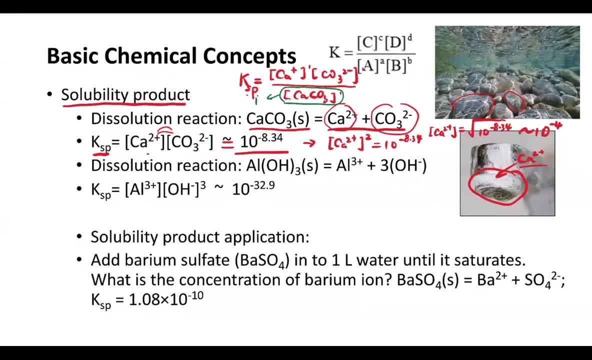 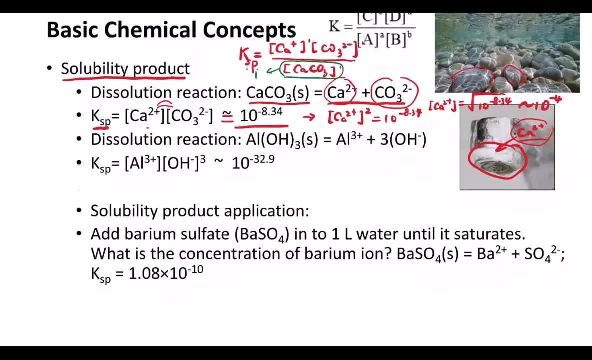 So this is also the reason why we have these trace amount of the calcium ions in our water. OK, so similarly, we can have the dissolution reaction of the aluminum hydroxide. So we know that aluminum hydroxide has a form of AL and this is aluminum. 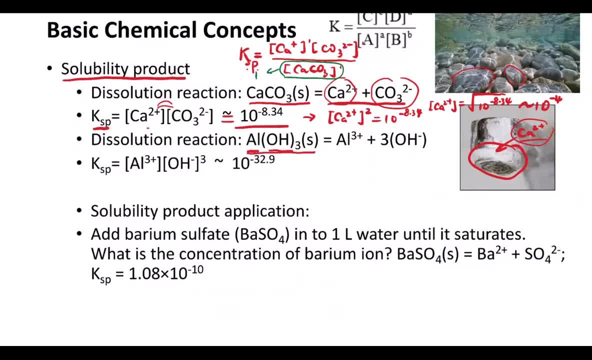 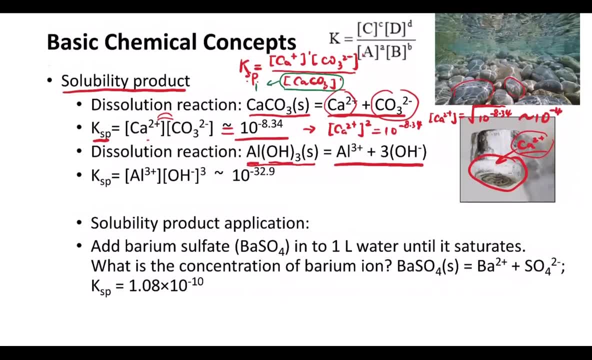 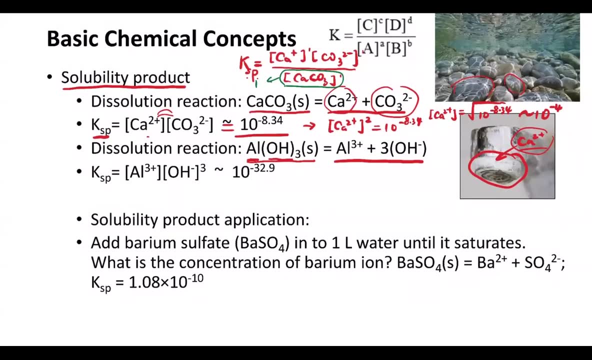 And it has three hydroxide ions. Right, And then they dissolve following this reaction. OK, So similarly, we can write out the equilibrium constant, or more specifically the KSP. OK, the solubility product. Again, we apply the concept that since this is a pure solid, so the term in the denominator should be equal to one. 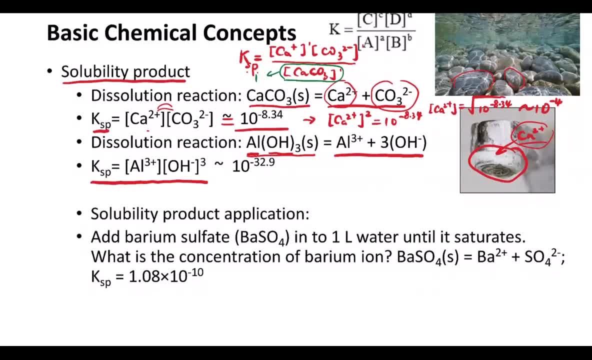 So that's why the KSP is equal to aluminum concentration multiplied by the OH concentration to the power of three Right. So it turns out that this solubility product is further very low value. This is extremely low: 10 to the negative 32.9.. 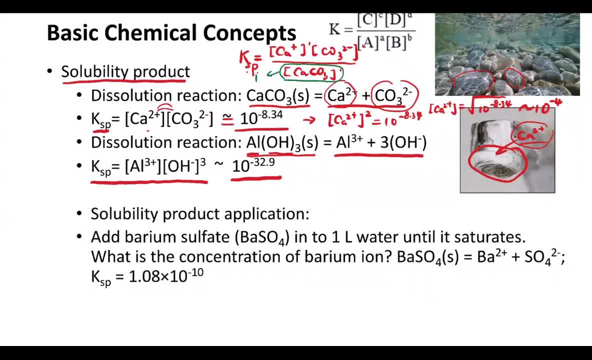 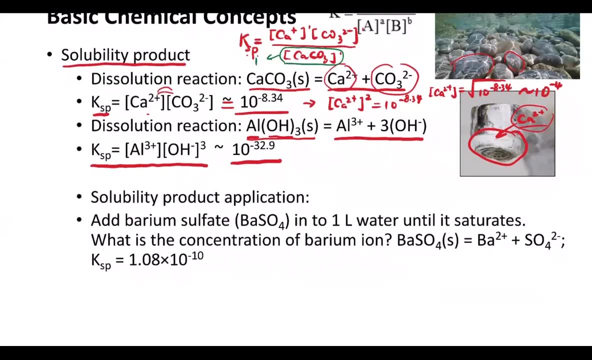 OK. so basically by using this concept here we can also calculate what is the concentration of the aluminum and what is the concentration of the hydroxide Right. So here I'm just going to give a very simple application Of this concept. 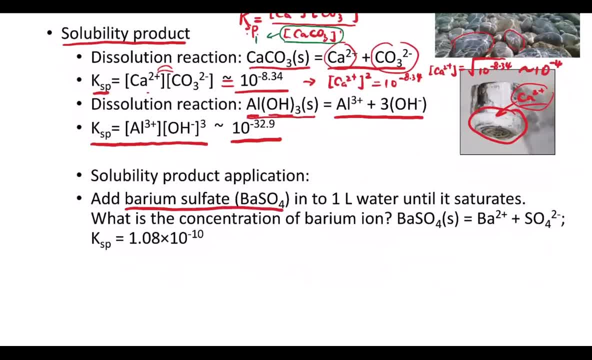 So let's say we're adding barium sulfate, which is a solid, into one liter of water until it saturates. What this means is that until the we cannot dissolve any more solid. OK, so what is the concentration of the barium ion? 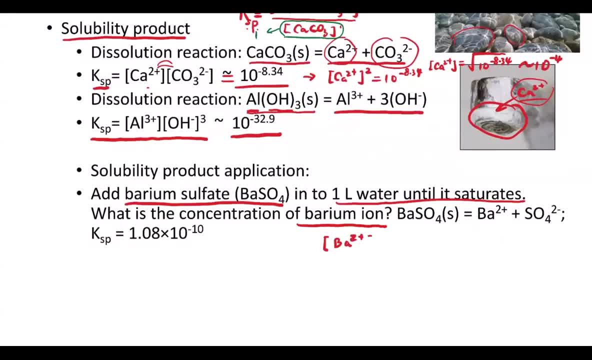 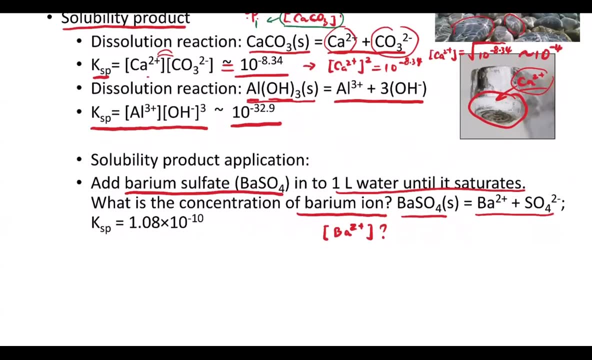 So basically it's asking for this concentration here. We know that the barium sulfate dissolves into barium ion and sulfate ion at a one to one ratio And we know the KSP is equal to 1.08 multiplied by 10, to the negative 10.. 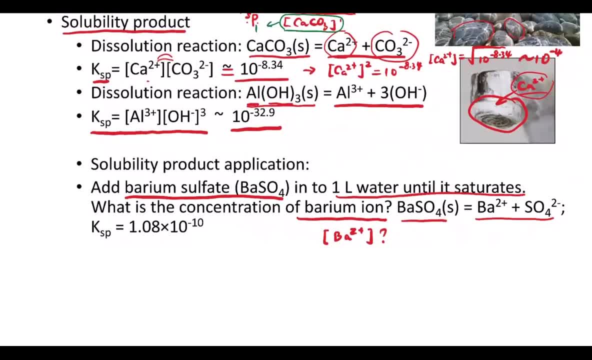 OK, So the way we solve this is similar to these ones. We can just write out the KSP, Right? So that's just barium ion concentration multiplied by. it's not carbonate ion, it's sulfate ions, Right? This value should be 1.08 multiplied by 10 to the negative 10.. 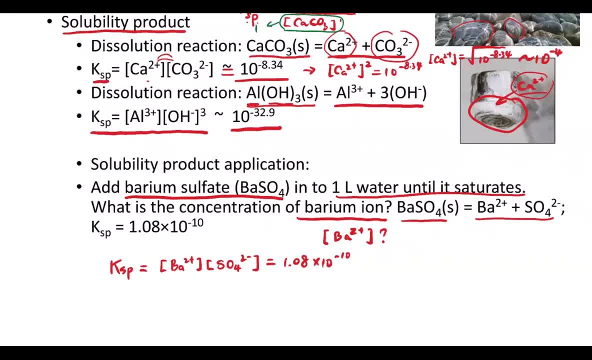 So further, since we're directly dissolving this salt in a pure water, right? So we know that, according to the stoichiometry, every one mole, or every one number of the barium ion is going to correspond with one number of the sulfate ion. 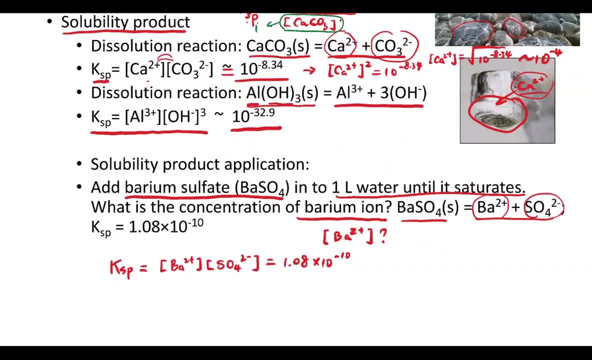 because there are no sulfate pre-existing in the water, Right. So that's why the barium ion concentration should be equal to the sulfate ion concentration. So because of that we have the barium ion concentration to the power of 2 equal to 1.08, multiplied by 10 to the negative 10.. 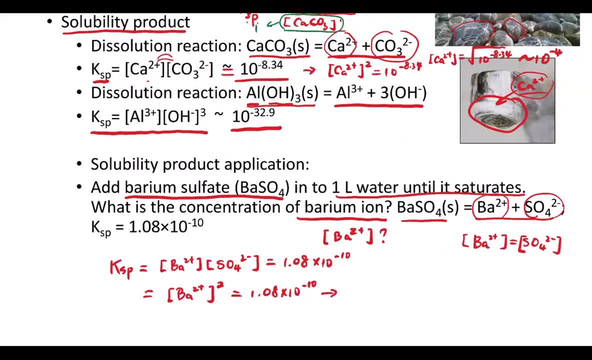 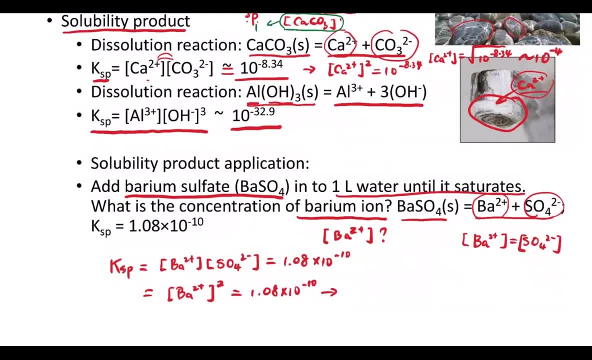 So further we can calculate. we can take the square root and then calculate the barium ion concentrations. So the things will be a little bit different. Let's say, if we add barium sulfate into one liter of the sodium sulfate solution. let's say, if we assume that the sodium sulfate concentration is 1m. 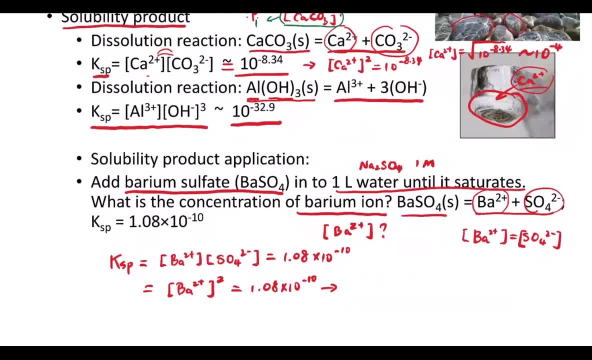 Okay. so what's going to happen? So, under this situation, we know that there are pre-existing sulfate ions in the water, right? So we cannot apply this relationship anymore. So what we should do is, basically, we know that, since there is already one mole per liter of the sulfate in the water, right? 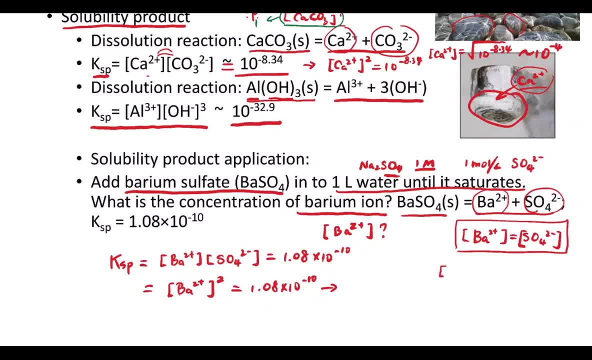 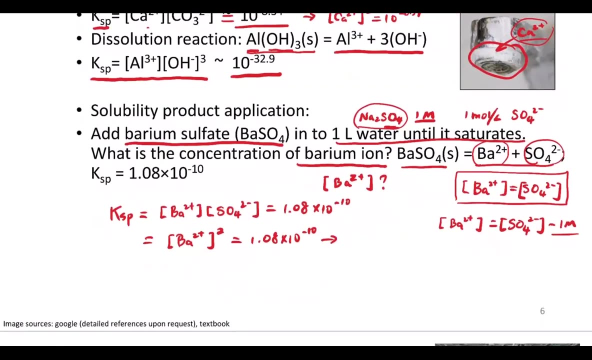 So we know that the, basically the barium ion concentration should be equal to the sulfate ion concentration minus 1m, right? So this 1m is coming from the sodium sulfate that's in the solution. So, under this situation, if it's not pure water, if it's 1m of the sodium sulfate, then this thing should become barium sulfate ions. 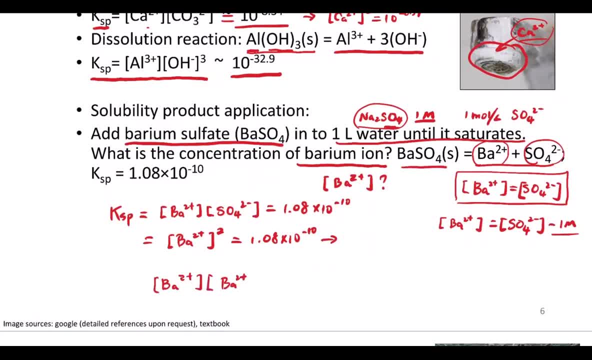 multiplied by the barium ion, sulfate barium ion plus 1, equal to 1.08. multiplied by 10 to the negative 10.. Okay, so instead of using this relationship, we're going to use this one, Because there is pre-existing 1m of sulfate in the solution, right? 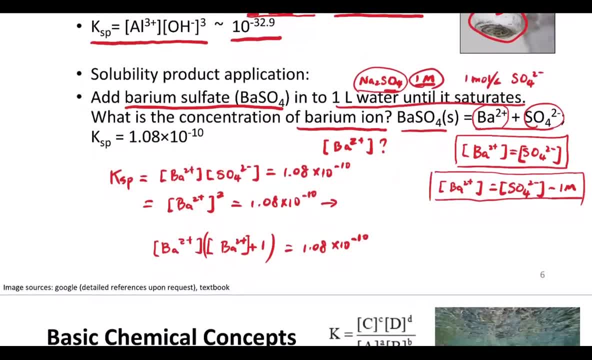 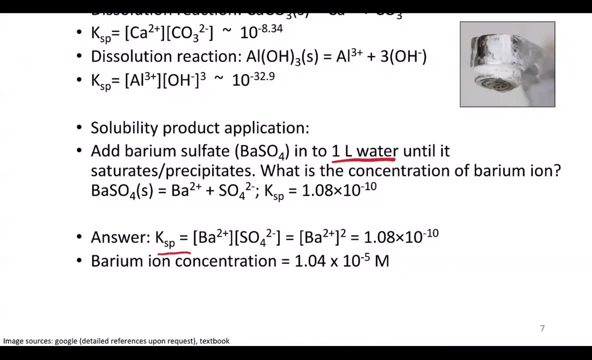 And then you can further solve this. So if you have this relationship, then you can find that the barium ion concentration will be further lower, actually significantly reduced, right? So if we just look at the water system, then we can just use this method. 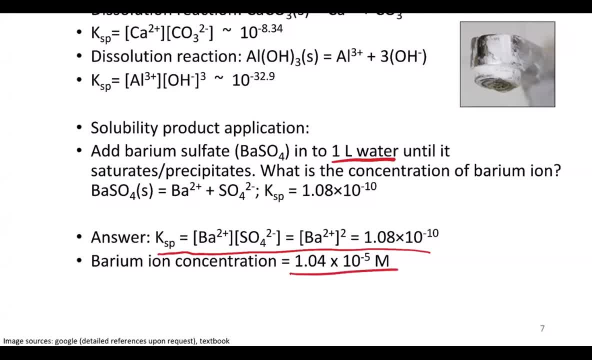 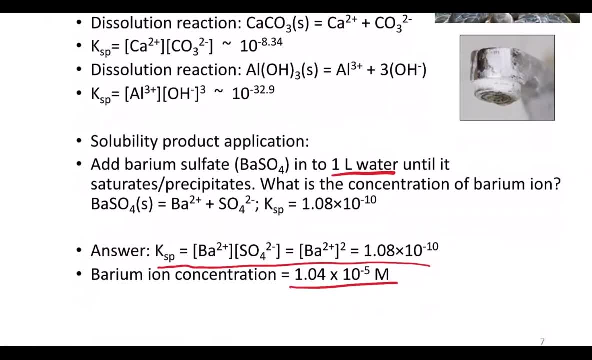 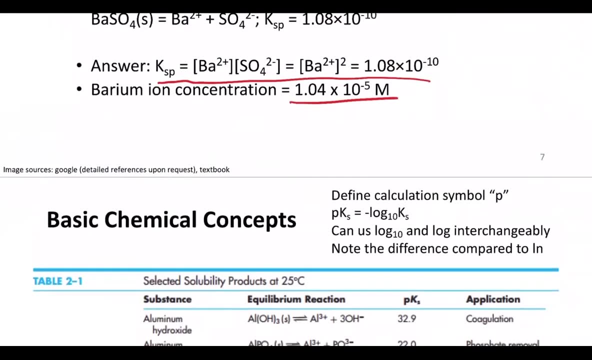 So it turns out that the barium ion concentration is 1.04 multiplied by 10 to the negative 5, which is a very low concentration, right? So this is an example for the for the solubility product. Okay so, but then you may wonder: where do we get all of these solubility product values? 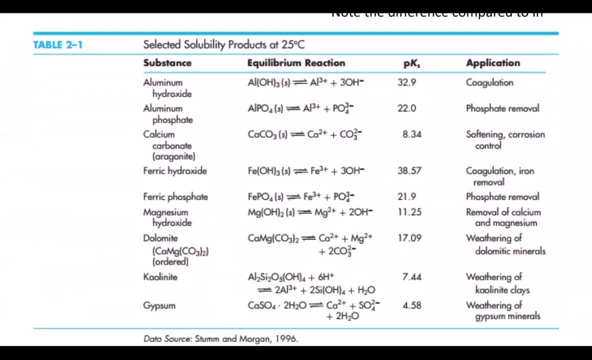 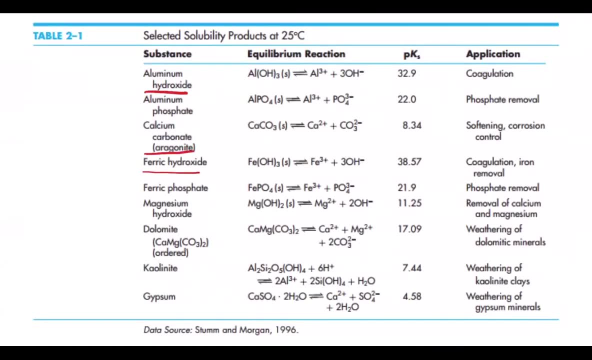 So in the textbook there is a table that's showing all of these common solids, For example, aluminum hydroxide, calcium carbonate, ferric oxide. right, So all of these came with this value of pks. Okay, so the pks is a way to show the solubility product. 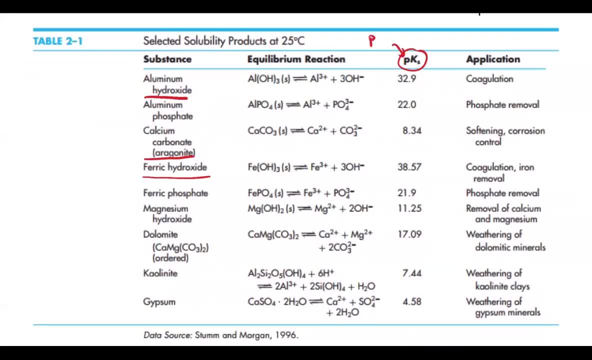 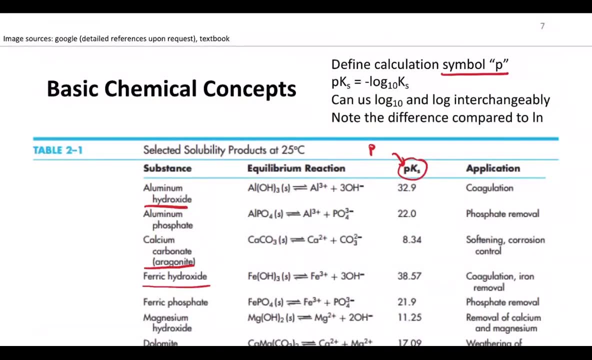 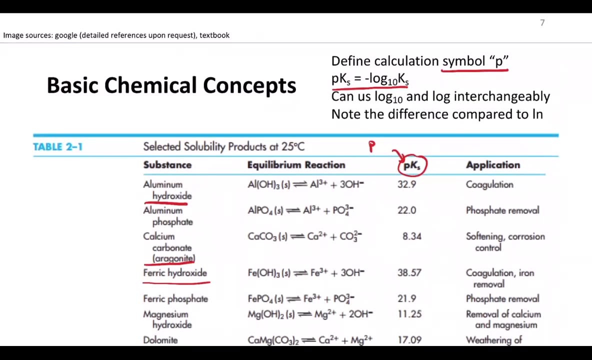 So you can think of this p here as a operator, Okay so as a type of calculation. So we define this calculation symbol, p, as pks equal to the negative log 10 of ks. Okay, So, basically the ks or the ksp. 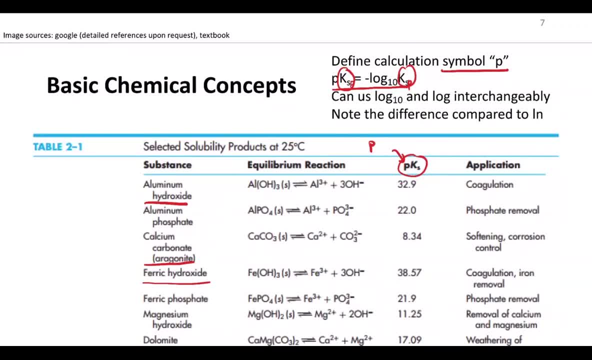 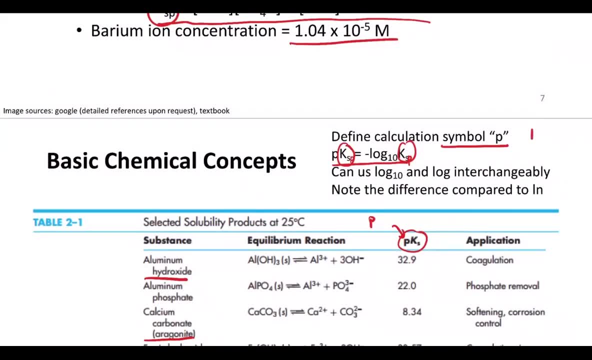 is a solubility product and the pksp or the pks is just negative. log 10 of this value, right. So for example, if we have a ksp that's equal to 10 to the negative 10, then the pksp. 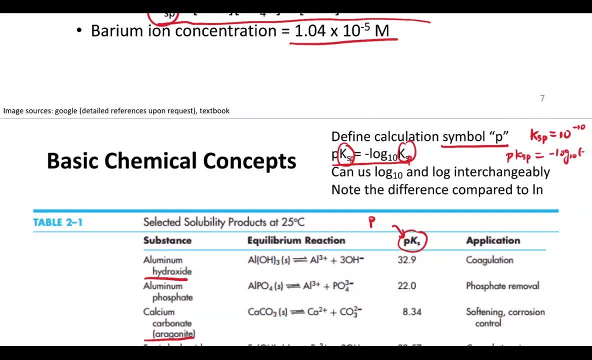 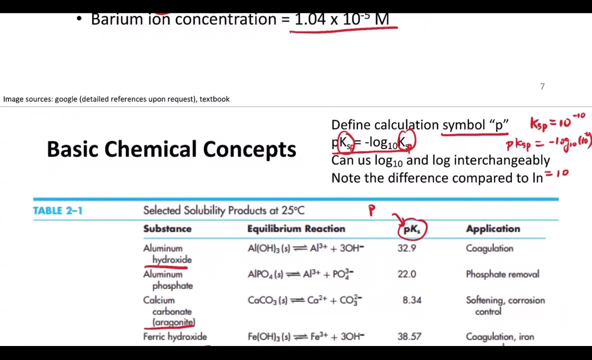 is just negative log 10 of negative log 10 of the of this thing here. Okay, so you're going to get a value of 10.. Right, So this is how we define this symbol p here. Okay, So what this means is that the higher or the larger the pks. 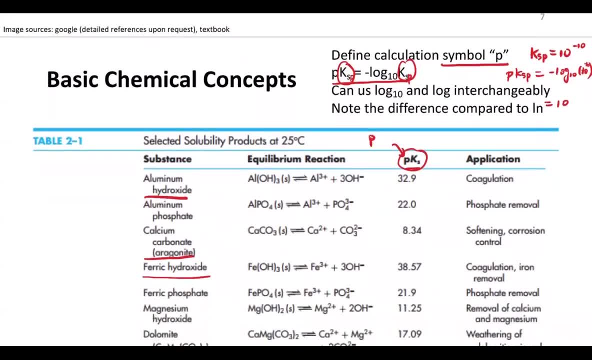 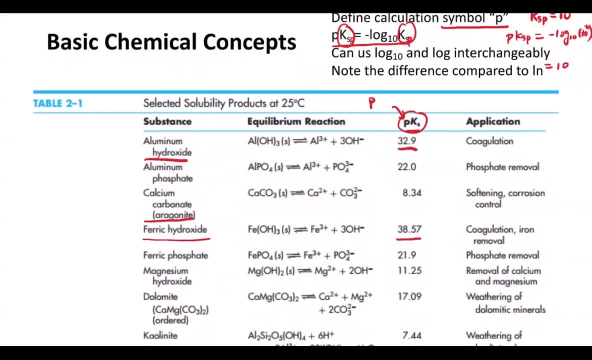 the more difficult to dissolve this solid right. So you can see the aluminum hydroxide has a very large value, right? The ferric hydroxide has a very large value, but compared to that, the calcium carbonate has a relatively lower value, which means that it's a little bit easier to dissolve this solid. 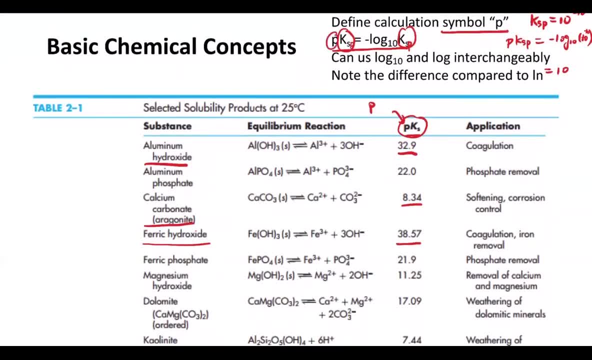 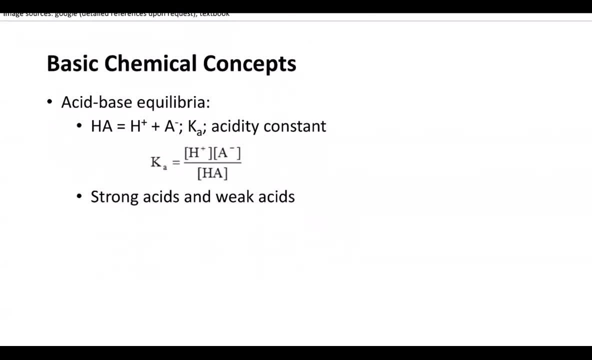 Okay, so we're going to come back to this operator p here again later on, Okay So, as I said, so one of the equilibrium is the precipitation dissolution equilibrium, where we introduce the solubility product. So another equilibrium is the acid-base equilibrium. 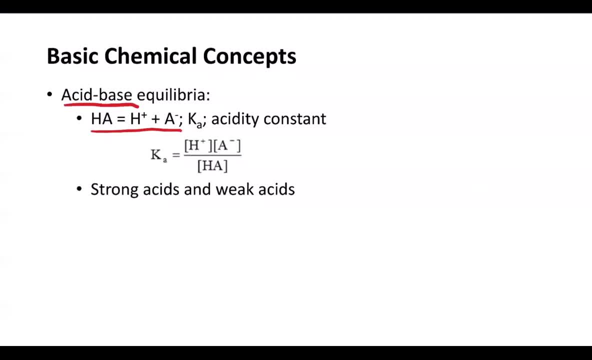 So what happens is that for any acid, they can dissolve into a hydrogen ion and some anion. Okay, so hydrogen ion is the cation and anion is the corresponding ion. For example, the hydrochloric acid is going to get dissolved into. 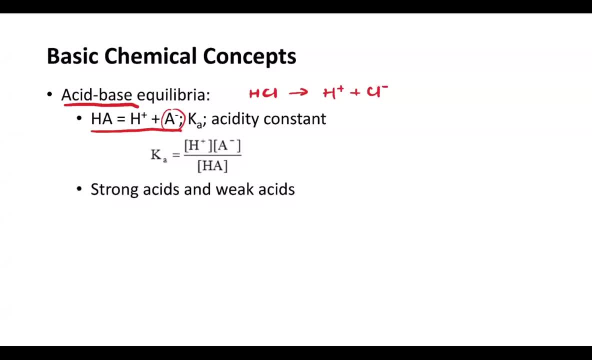 the hydrogen ion or the proton ion and the chloride ion, right, So this A here is just chloride ion. So for any of these dissolution of the acid, then we can also define a equilibrium constant, Ka. Okay, so following the definition of the equilibrium constant, 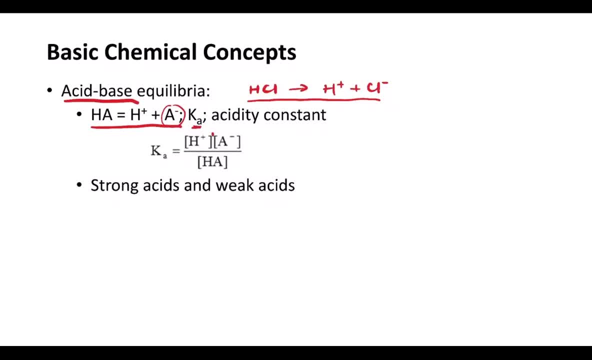 then it should be the concentration of the proton ion to the power of one, the concentration of the anion to the power of one, and divide by the concentration of the acid. Okay, so because of that you can have very strong acids or very weak acids. 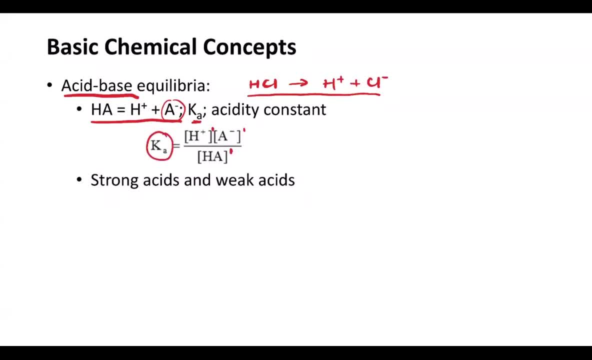 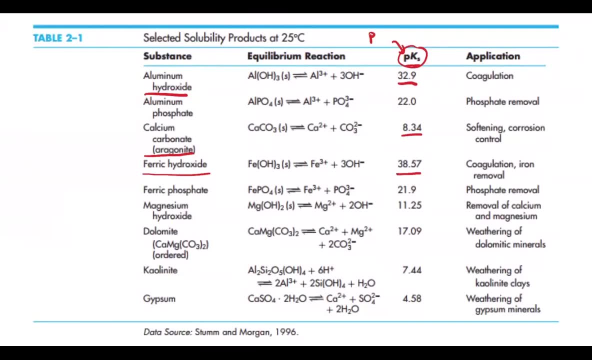 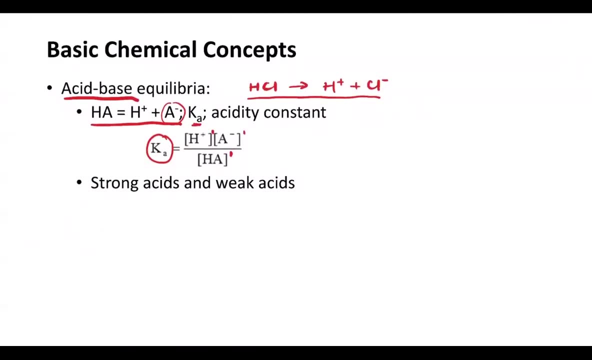 So that's shown in this equilibrium constant here. So if you recall, in here we mentioned that the larger the PKS, then the more the difficult it is to dissolve these solids, right? So the same thing happens to these acids or these base. 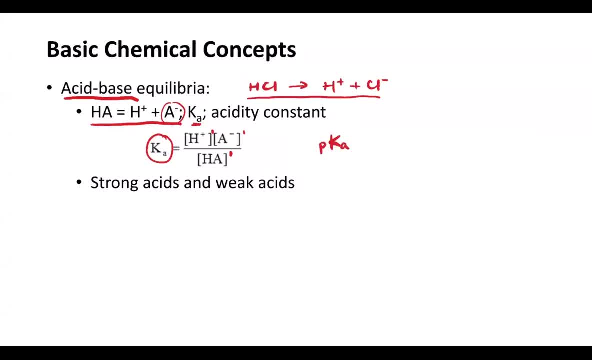 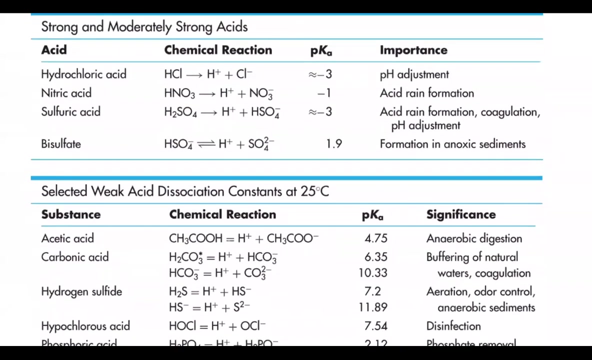 So we can also define the value, define the calculation, PKA. So what this means is the higher the value, the more difficult to dissolve. So the more the difficult to dissolve, then the weaker the acid right. So here we have a table that's showing the PKA values of common acids. 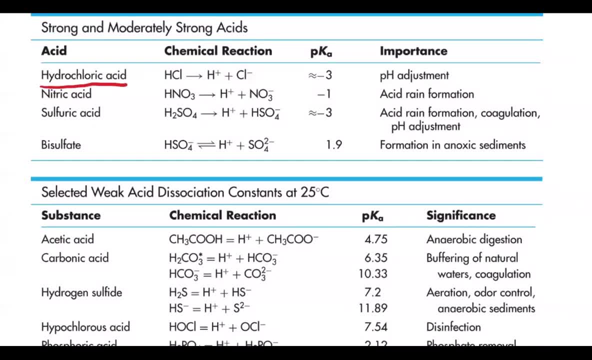 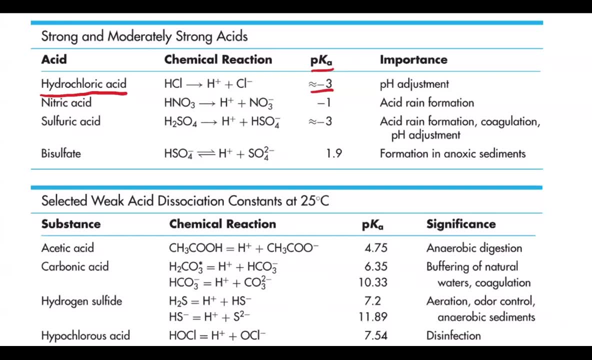 You see that the strong acids, they have such a low value of the PKA that some of them even go to negative three. Okay, so a value of negative three means that the, basically the KA value is equal to 10 to the third. 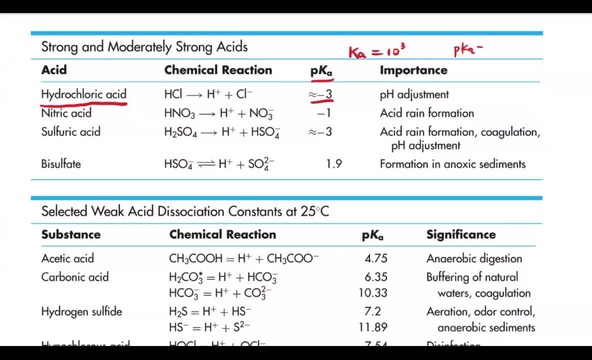 right. So, if you recall, the PKA is equal to negative log 10 of KA, right? So if you have a KA value of 10 to the third, then this is going to be negative three. Okay, so if you have a very large, 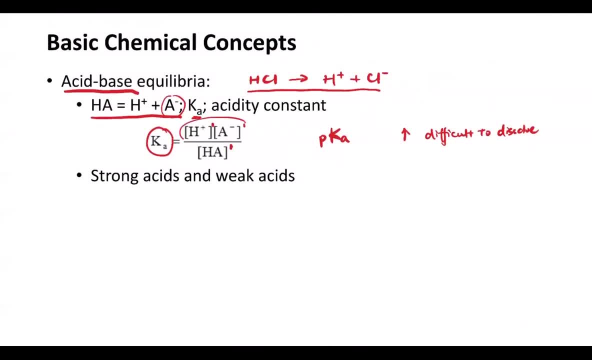 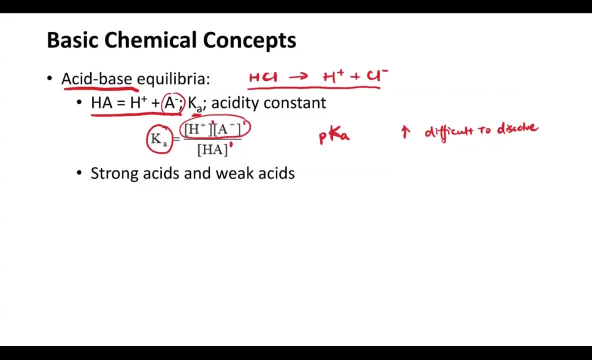 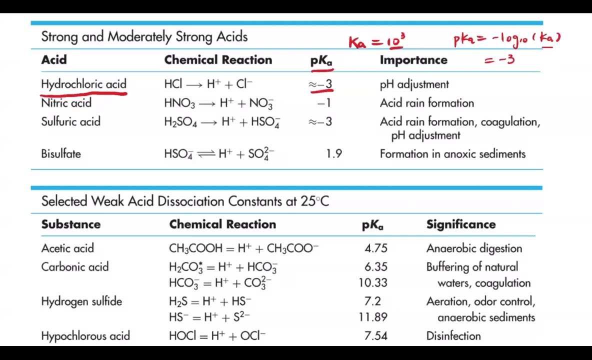 very small PKA value. it just means that the concentration of the proton ions multiplied by the concentration of the ion is much, much higher compared to the remaining acid concentration. So that's why the strong acids will have a very small value of the PKA. 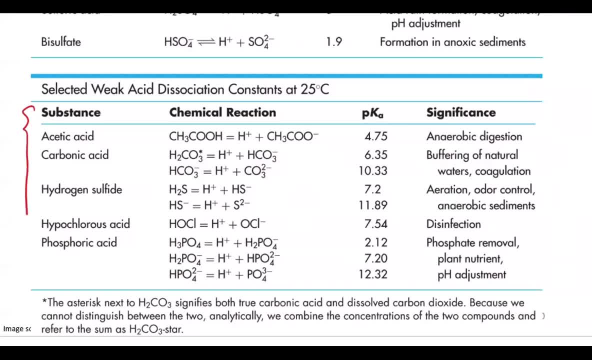 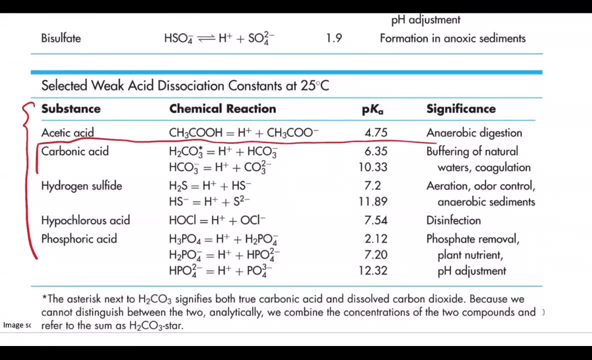 while the weak acids are going to have larger values of the PKA. So here a very important system is the carbonic acid, because in the atmosphere there are carbon dioxide existing in the system right. So the carbon dioxide once they dissolve into the water. 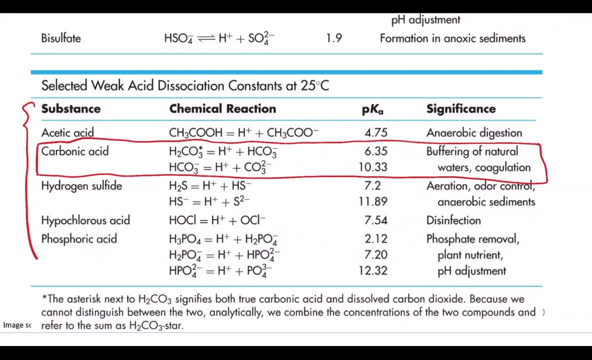 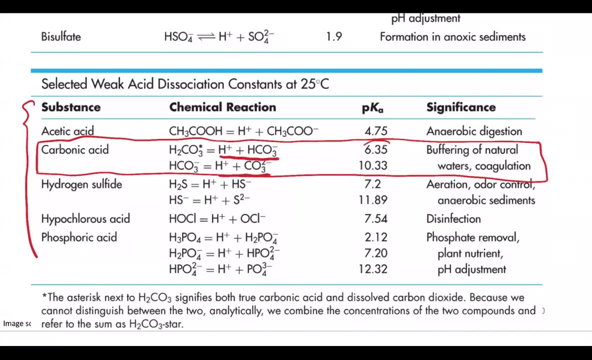 they can form carbonic acid and further get dissolved into the proton and the bicarbonate ion, and further the bicarbonate ion can dissolve into proton ion and the carbonate ions. right So for these two reactions, as you can see, they have a pretty large PKA value. 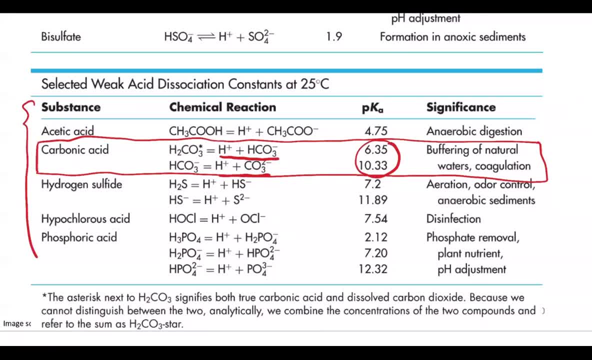 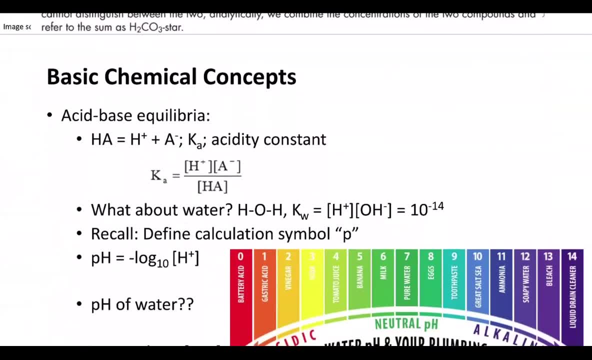 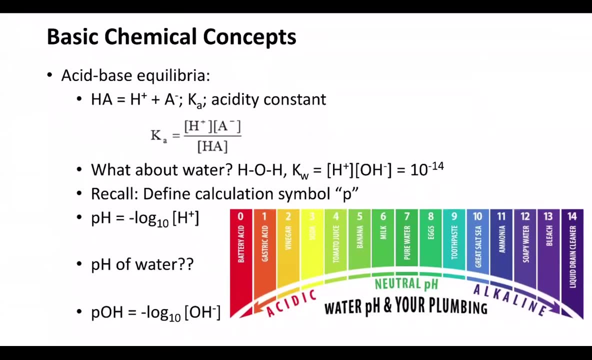 which means that they are weak acids. The concentration of these proton ions are going to be lower in the system, right? So then, a very easy application is the water. Okay, So what about water system? We know that water can be written as H connected to an O. 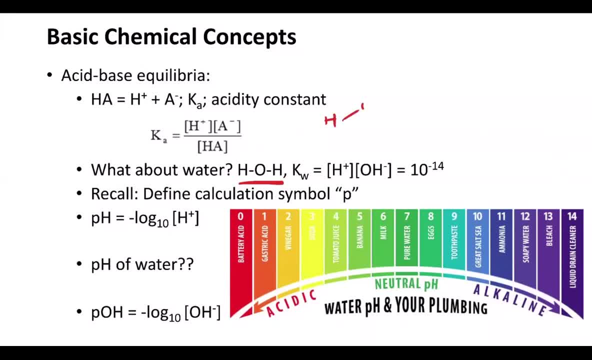 oxygen and further and hydrogen. right, We know it's composed of this structure. Okay, So water, you can treat it as a very weak acid. Okay, So basically the water or the hydrogen here they can get dissolved into, get dissolved into the water. 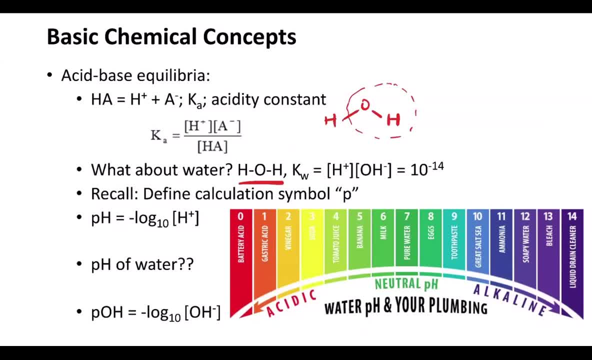 right To form the protons. So for this reaction here we can also. so basically, water is getting dissolved into proton and the hydroxide ion. So for this reaction we can also write out its equilibrium constant right. So that's going to be. 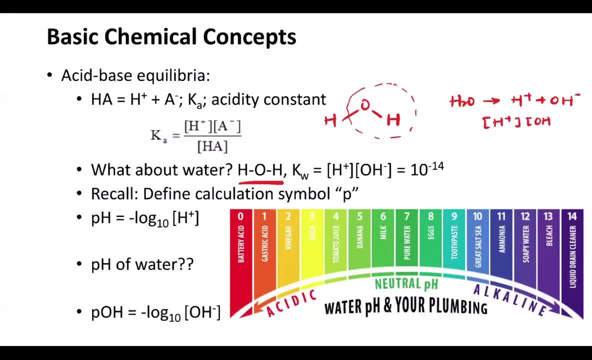 hydrogen multiplied by OH, divided by the concentration of water. So, if you recall the note, that's earlier. so for pure liquid, this term should be regarded as one. Okay, So that's why we can define a equilibrium constant for water: Kw. 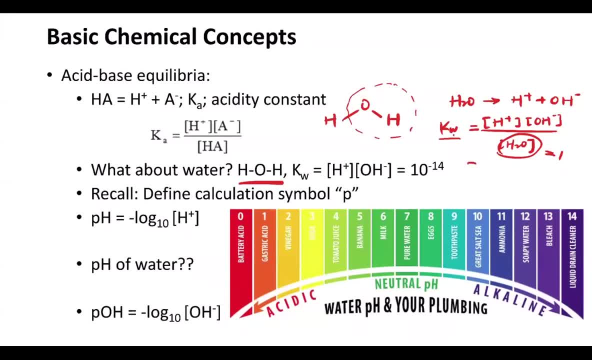 W stands for water here. Okay, So that turns out to be 10 to the negative 14.. So people have done these measurements All right. So now, if you imagine we have a cup of water, let's say it's just water inside. 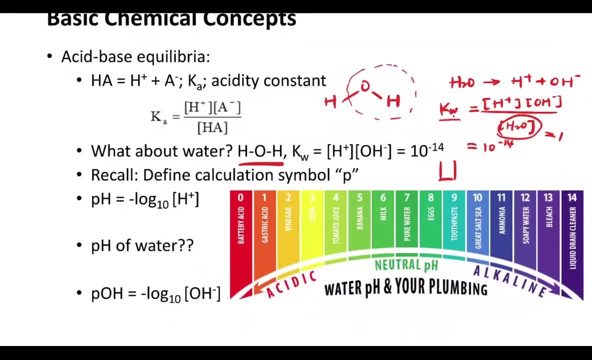 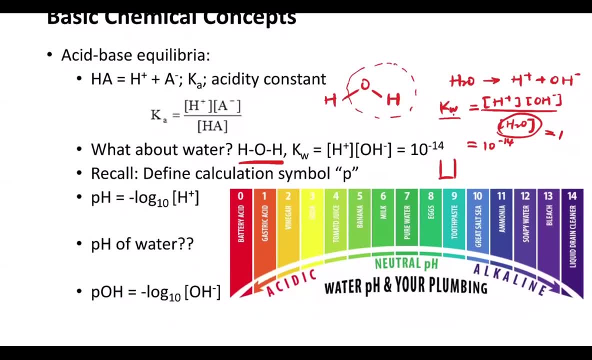 It doesn't have any ions inside right. And then let's see what's the concentration of the hydrogen and OH. So what happens is they're going to dissolve at a molar ratio one to one right. So basically, the concentration of hydrogen ions is going to be 10 to negative 7,. 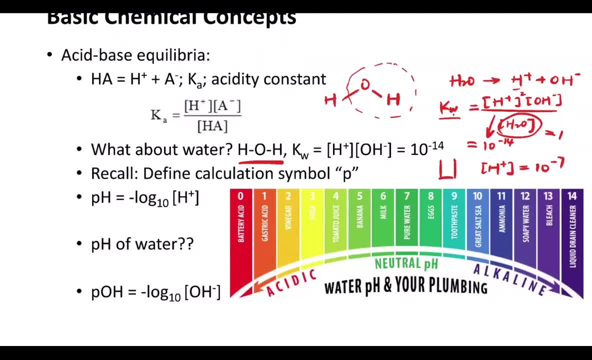 because basically this is going to be squared because these two are the same right, And then you can solve that So further. let's again use the definition of the P. So let's say we have the pKa, pKs.